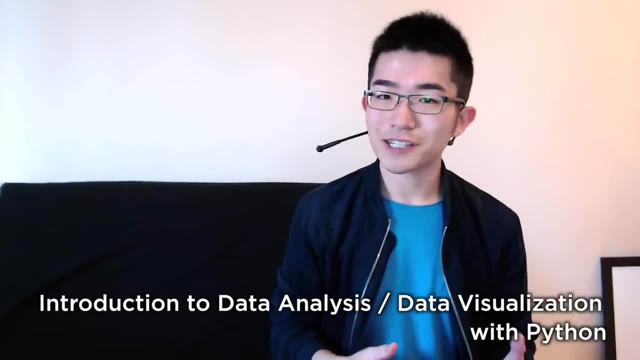 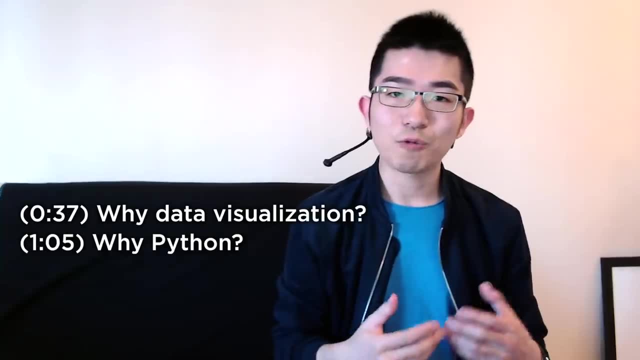 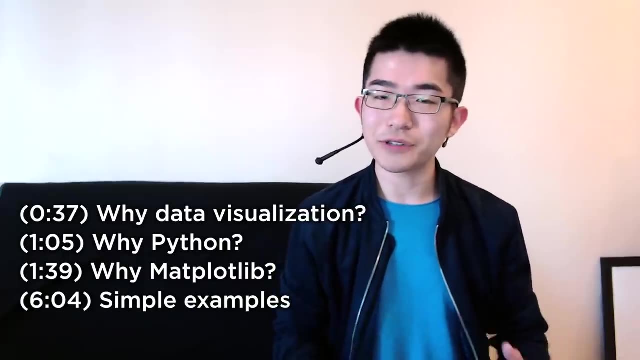 Hey everyone, this is my introduction to data analysis slash data visualization with python. In this video, I'm going to cover why you might want to use data visualization and why you might want to use python and matplotlib for it, And then we're going to go over some simple examples of how to actually use these tools. 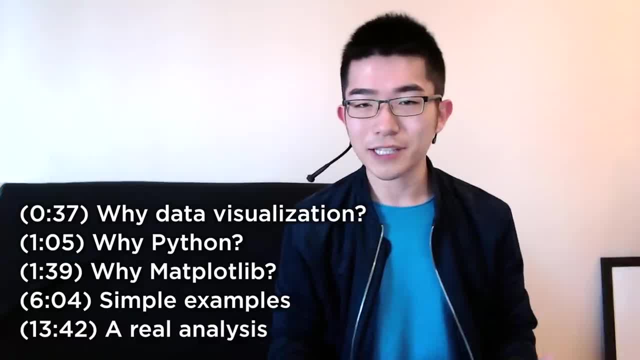 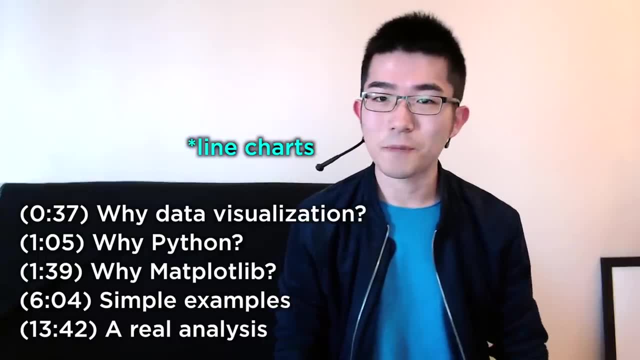 And then, using these tools, we're going to do sort of a real analysis with a real dataset at the end, And in this video I'm only going to cover line charts. just to keep everything simple, I'm also going to put a more detailed version of this outline in the comment section below. 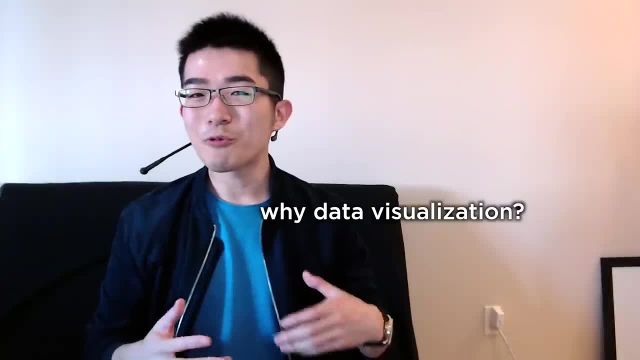 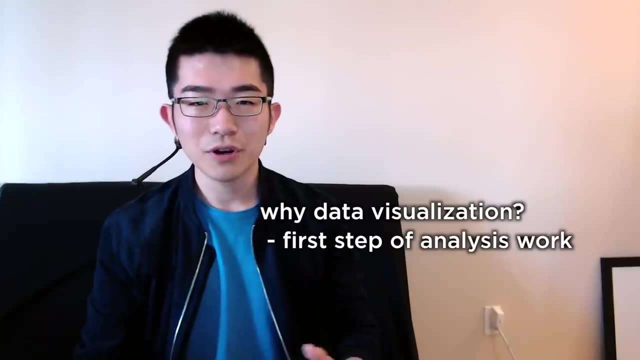 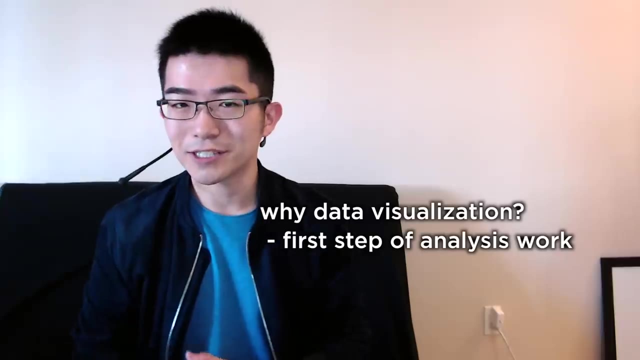 so you don't have to watch the whole thing if you don't want to, Okay, so why should you use data visualization in the first place? Well, data visualization is actually often the first step of any type of data analysis work, whether it's simple data analysis or statistical analysis, or machine learning analysis. 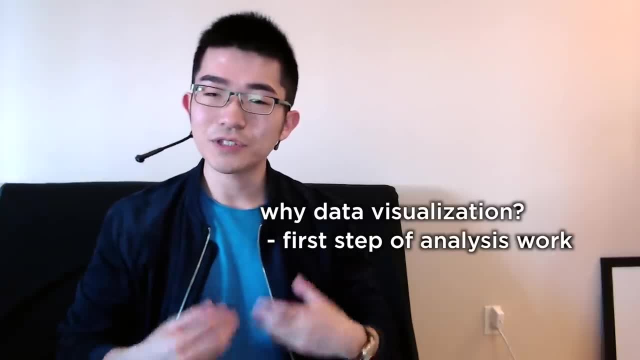 And the reason for that is because visualizing data often gives you an intuitive understanding of the data And it often helps you to understand the data better. And it helps you to understand the data better. And it helps you to understand the data better. 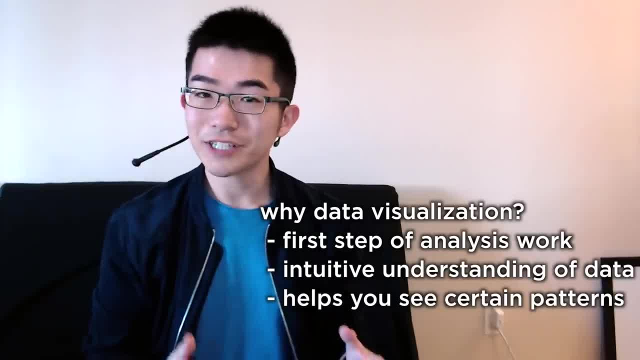 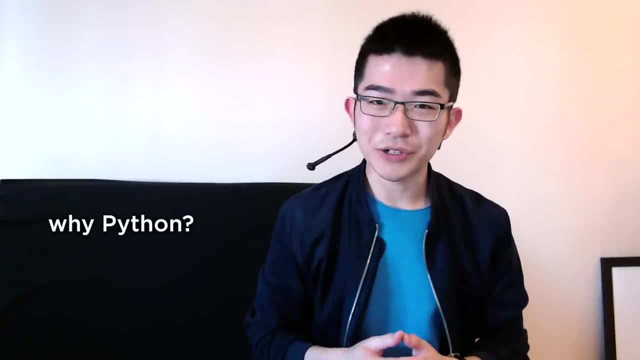 And it helps you see patterns that are otherwise hard to see, And we're going to see an example of that later. Okay, and why should you use Python for this? Well, Python is not the only good choice, but I would say it's one of the best. 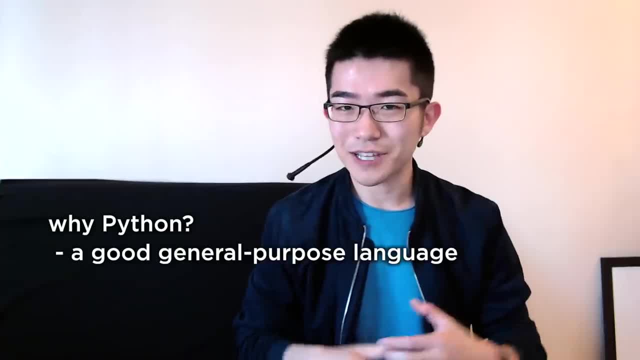 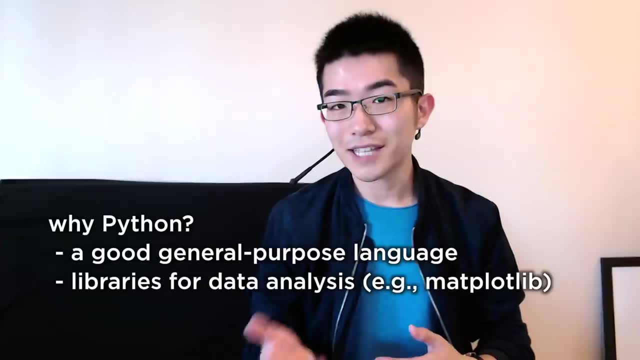 And the reason is, first of all, it's a general purpose language that's pretty easy to use and learn, And it also has many libraries for scientific computing and data science, including Mapple lib, And if you work at a company, your company might already use Python for something else. 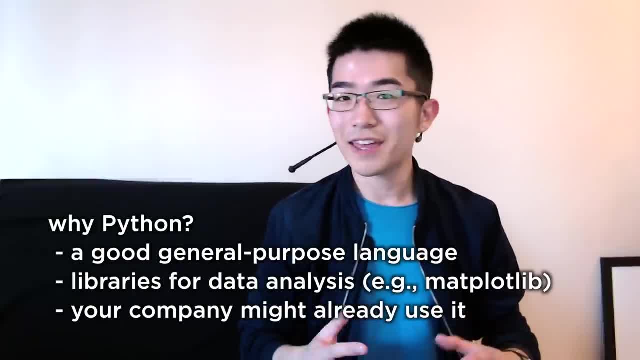 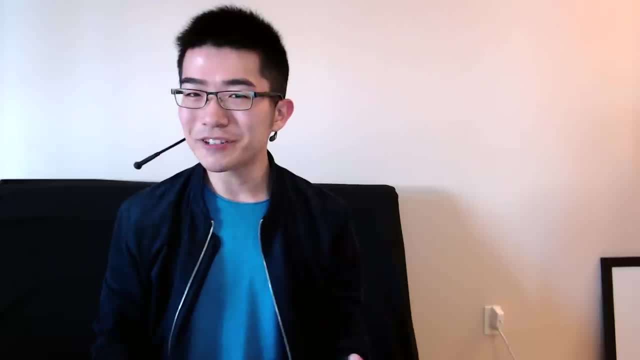 And if that's the case, that's really nice, because then you and your team are not going to have to learn a totally new language to do some data analysis. And why are we using Mapple lib for this? Well, Mapple lib is not the only good visualization library for Python. 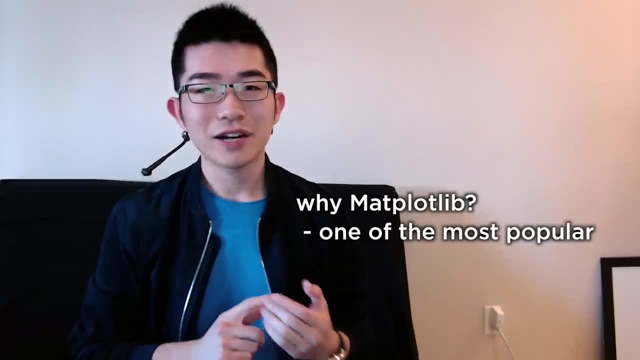 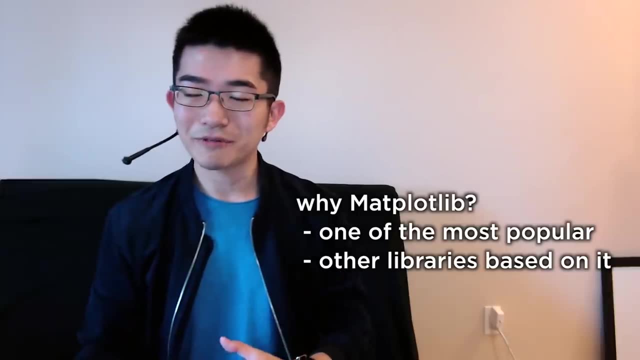 but it's still one of the most popular choices, And there are actually other libraries that are based on Mapple lib. So if you learn Mapple lib, it's going to help you learn these other libraries, For example, this one called Seaborn later on, if you want to. 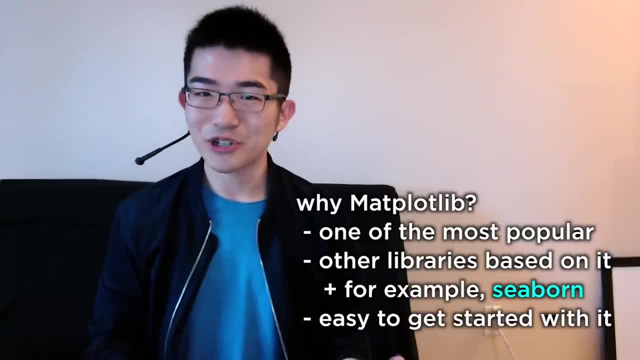 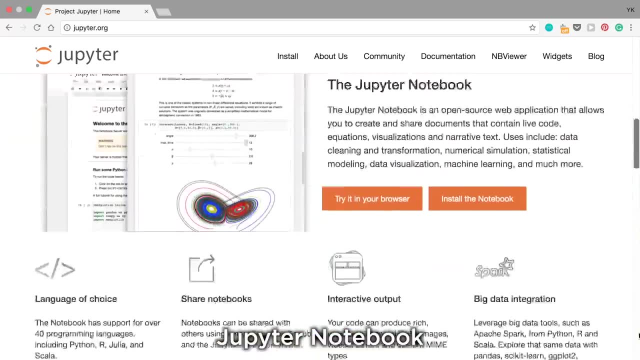 And Mapple lib is also pretty easy to get started with. Anyway, let's dive into a demo. For this demo, we're going to use something called Jupyter Notebook and a few other Python libraries, and we're going to use Anaconda to install them. 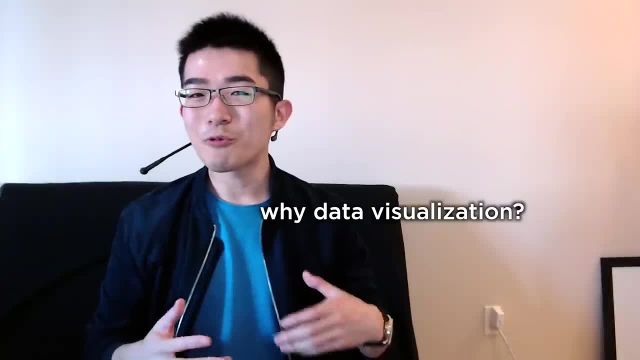 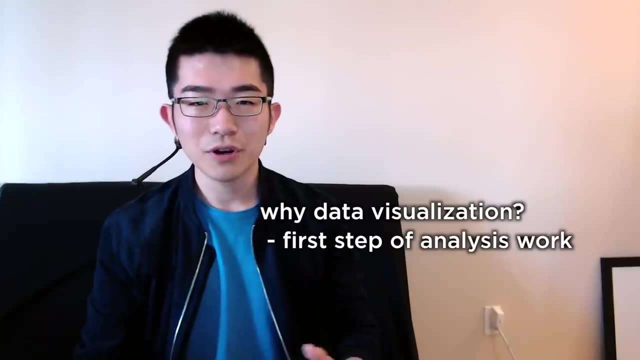 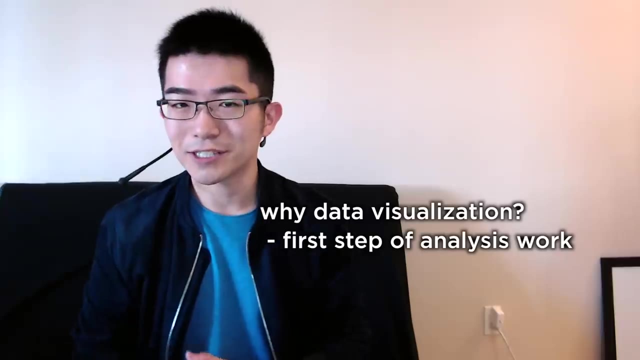 so you don't have to watch the whole thing if you don't want to, Okay, so why should you use data visualization in the first place? Well, data visualization is actually often the first step of any type of data analysis work, whether it's simple data analysis or statistical analysis, or machine learning analysis. 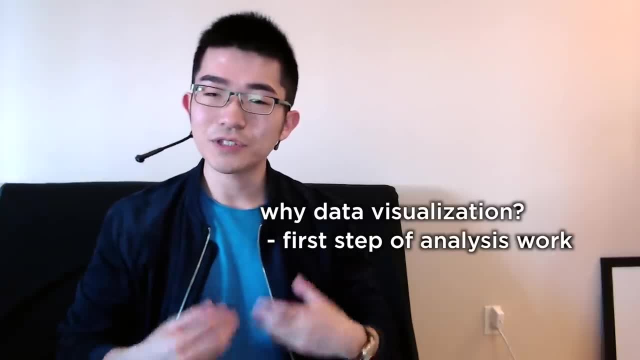 And the reason for that is because visualizing data often gives you an intuitive understanding of the data And it often helps you to understand the data better. And it helps you to understand the data better. And it helps you to understand the data better. 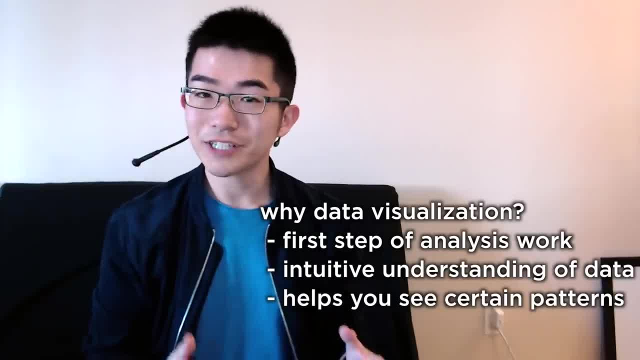 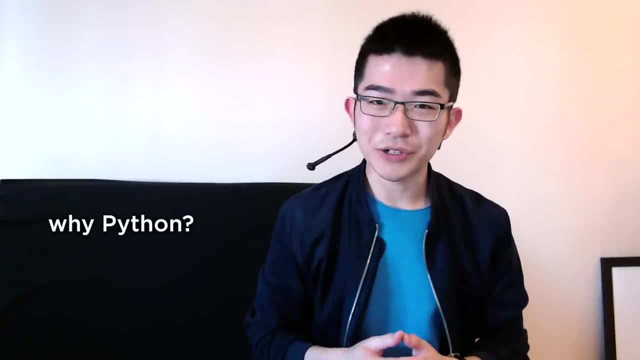 And it helps you see patterns that are otherwise hard to see, And we're going to see an example of that later. Okay, and why should you use Python for this? Well, Python is not the only good choice, but I would say it's one of the best. 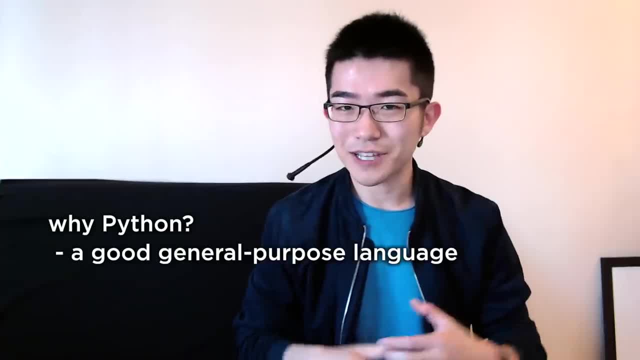 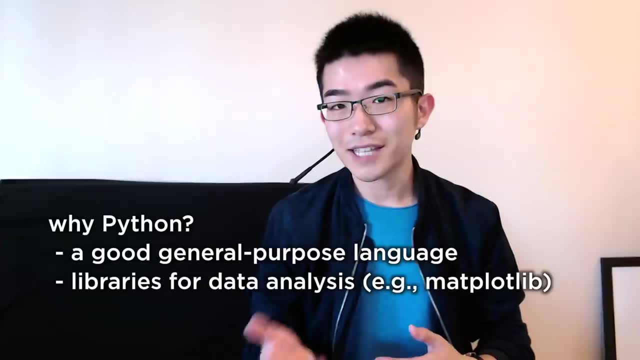 And the reason is, first of all, it's a general purpose language that's pretty easy to use and learn, And it also has many libraries for scientific computing and data science, including Mapple lib, And if you work at a company, your company might already use Python for something else. 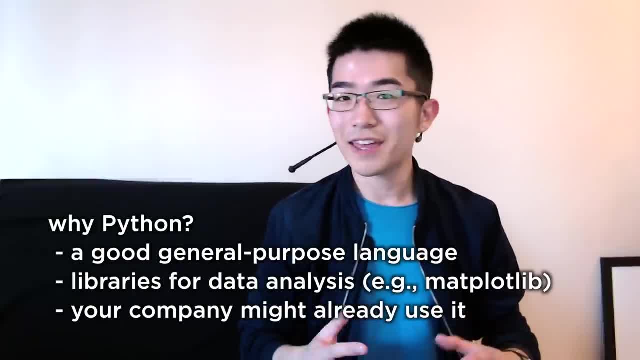 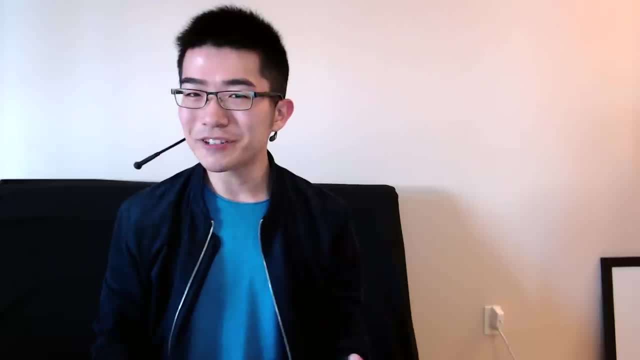 And if that's the case, that's really nice, because then you and your team are not going to have to learn a totally new language to do some data analysis. And why are we using Mapple lib for this? Well, Mapple lib is not the only good visualization library for Python. 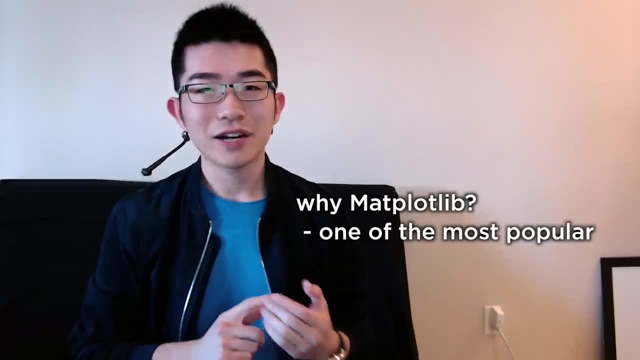 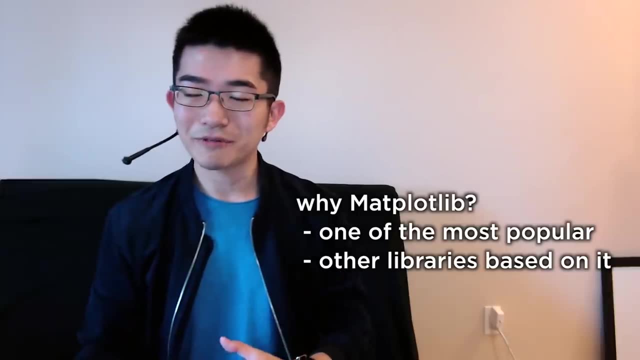 but it's still one of the most popular choices, And there are actually other libraries that are based on Mapple lib. So if you learn Mapple lib, it's going to help you learn these other libraries, For example, this one called Seaborn later on, if you want to. 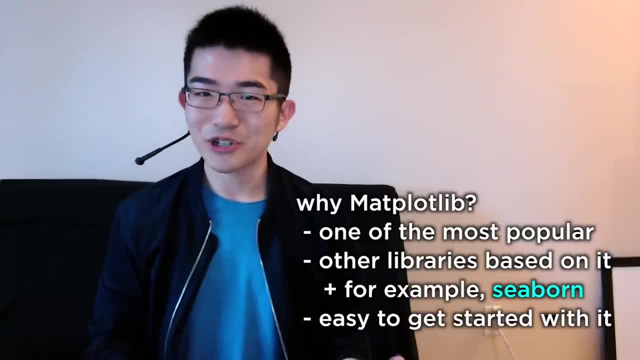 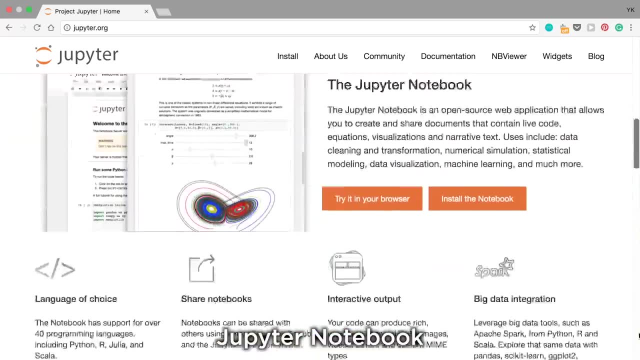 And Mapple lib is also pretty easy to get started with. Anyway, let's dive into a demo. For this demo, we're going to use something called Jupyter Notebook and a few other Python libraries, and we're going to use Anaconda to install them. 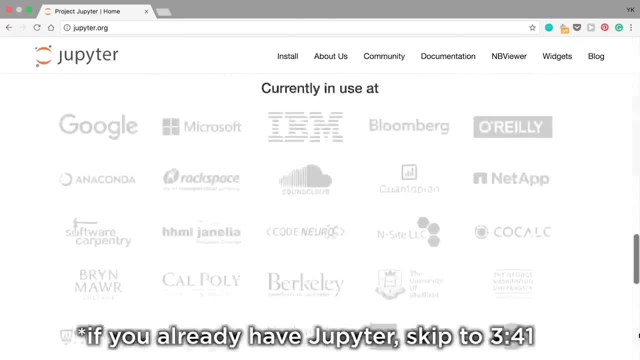 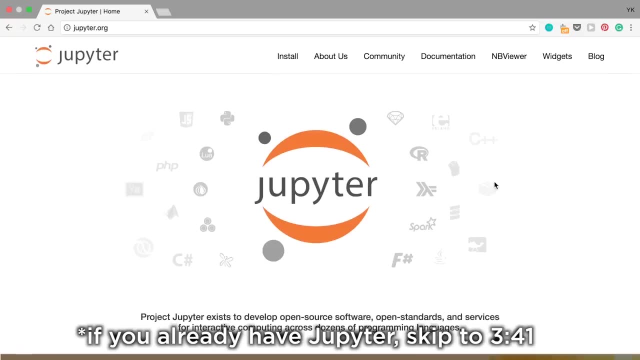 If you're not familiar with Jupyter Notebook and Anaconda, I have an explanation about them in my Python tutorial video, So I'm going to leave a link to that in the description. Anyway, to install Anaconda, just search for Anaconda Python. 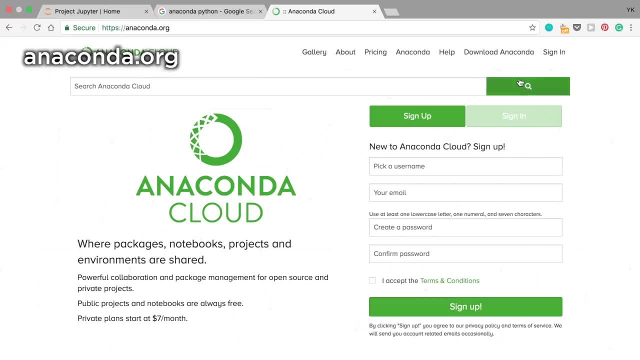 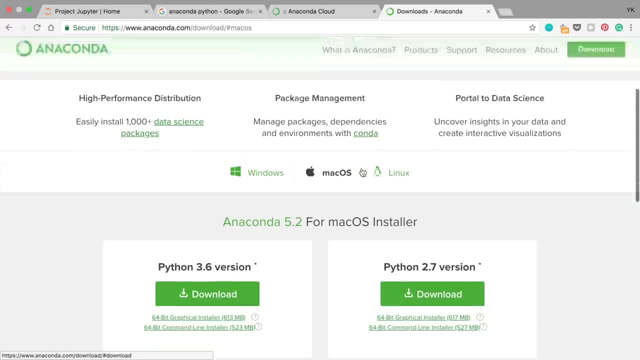 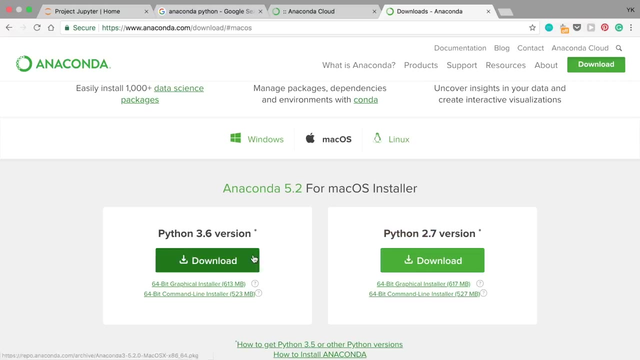 or directly go to Anacondaorg and there find the button that says Download Anaconda and select whatever OS you're using- I'm using Mac here- and click Download under Python three point something version instead of Python two point something, because we're going to use Python three here- and select where you want to. 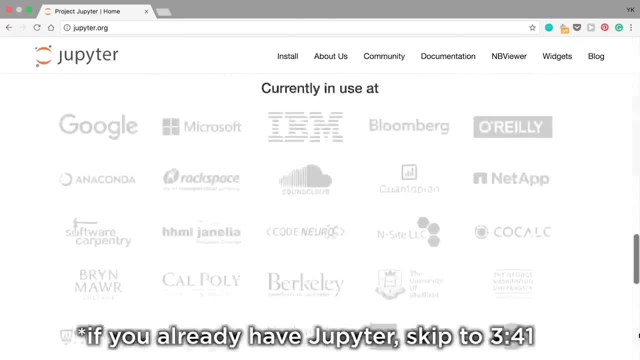 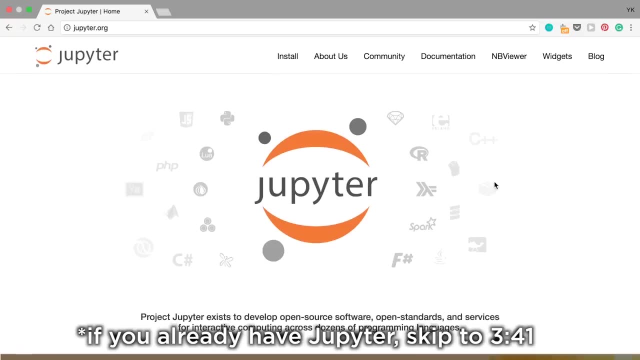 If you're not familiar with Jupyter Notebook and Anaconda, I have an explanation about them in my Python tutorial video, So I'm going to leave a link to that in the description. Anyway, to install Anaconda, just search for Anaconda Python. 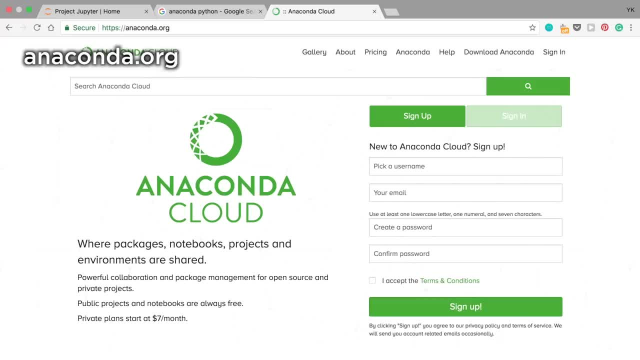 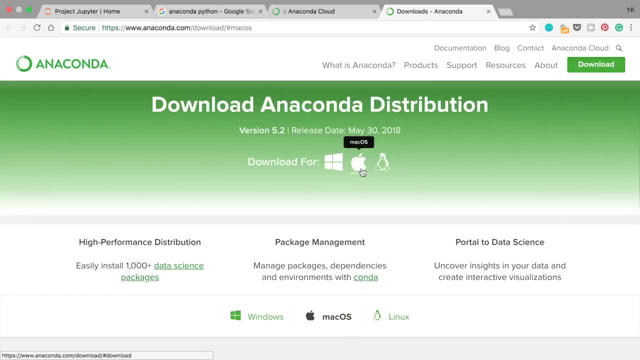 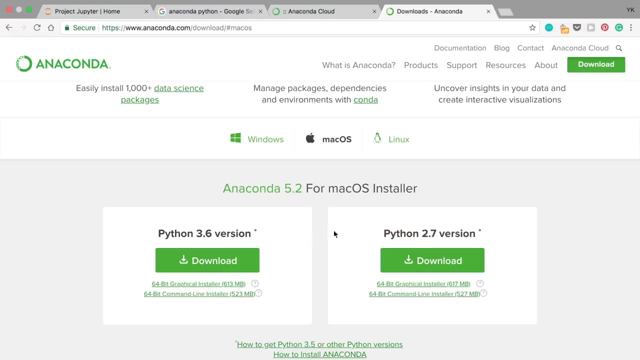 or directly go to Anacondaorg and there find the button that says download Anaconda and select whatever OS you're using- I'm using Mac here- and click download under Python three point something version instead of Python two point something, because we're going to use Python three here and select. 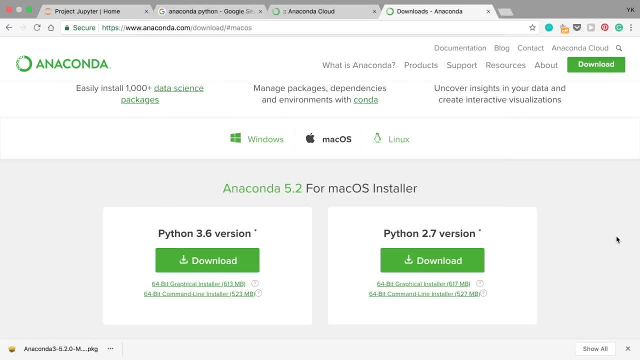 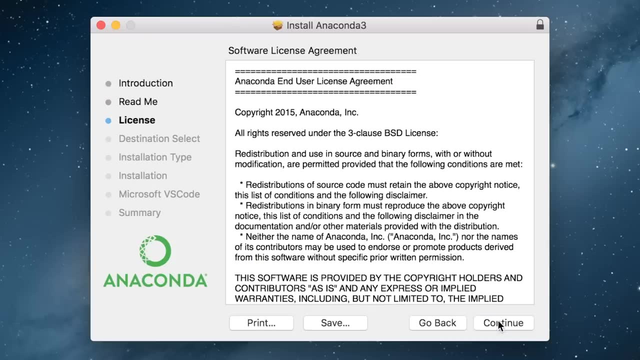 where you want to download this package, save it And, once it's downloaded, open up the package that you just downloaded and then just click continue, Continue, continue, continue, continue. agree. install for me only or install on a specific disk. 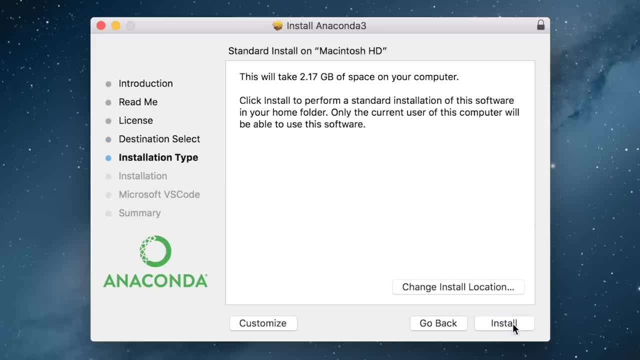 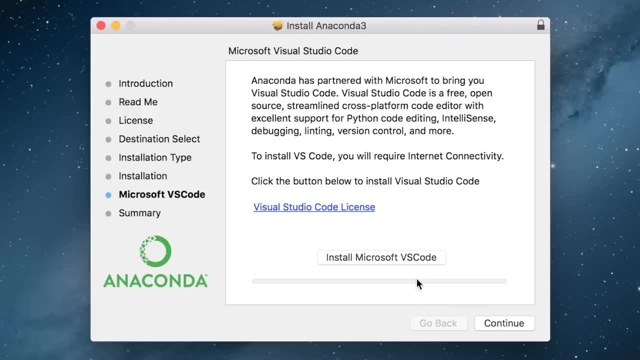 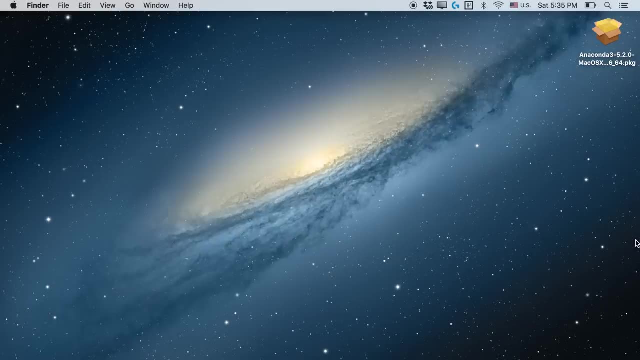 It doesn't matter which one, and continue and click install. And this process is going to take a while. After some waiting, you might see this prompt to install Microsoft VS code. We don't need that, So let's just continue here and then close, and then to launch Jupyter Notebook, you can. 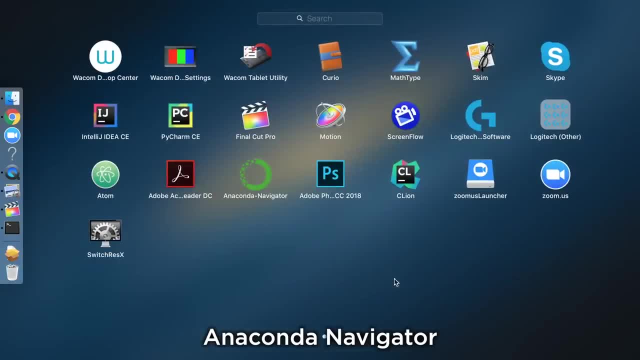 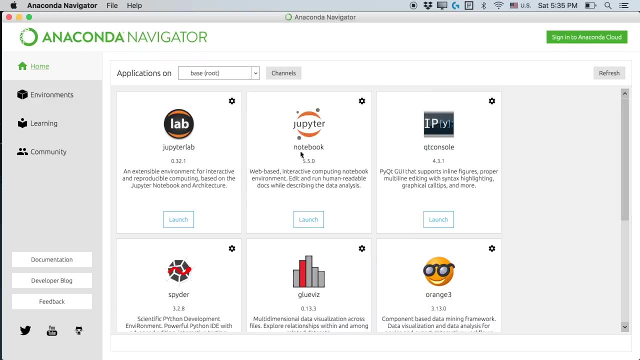 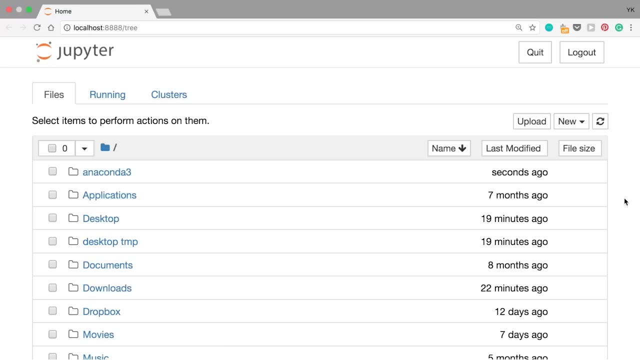 do it through this thing called Anaconda Navigator. So just launch it Like you launch any other application, just dismiss whatever comes up and then click launch in the Jupyter Notebook section, And then you should see a browser window show up with the Jupyter Notebook interface. 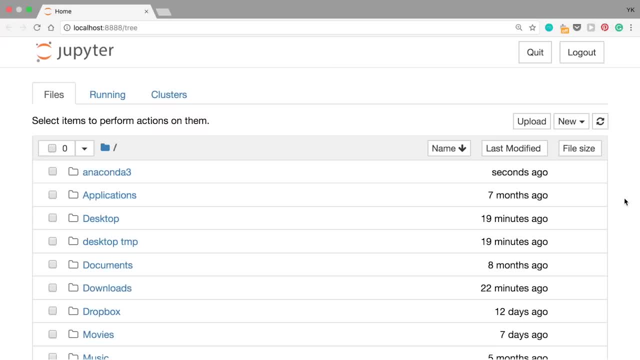 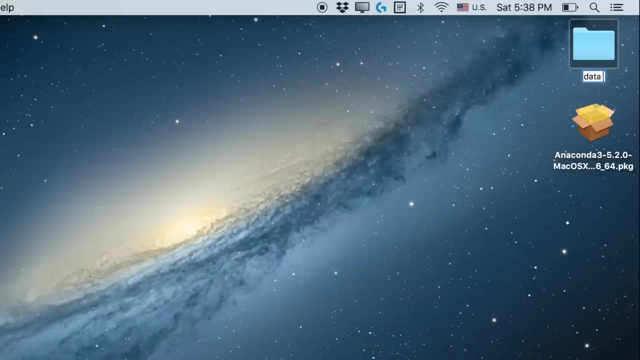 Now, if you want to follow this tutorial, the first thing you should do is you should create a new folder, Let's say on desktop, and let's call this one data visualization, and we're going to put all our data. So we're going to go to the Jupyter Notebook file here. 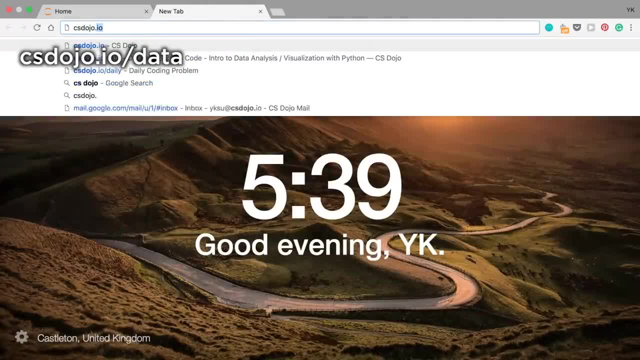 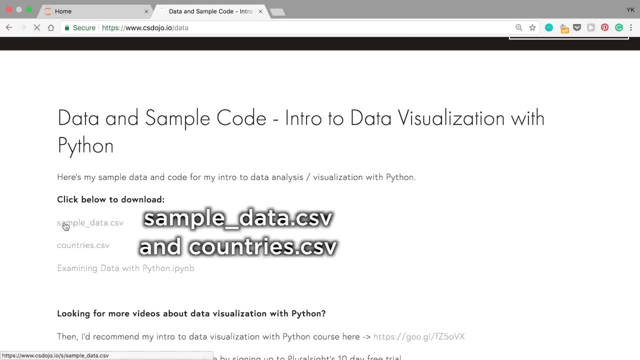 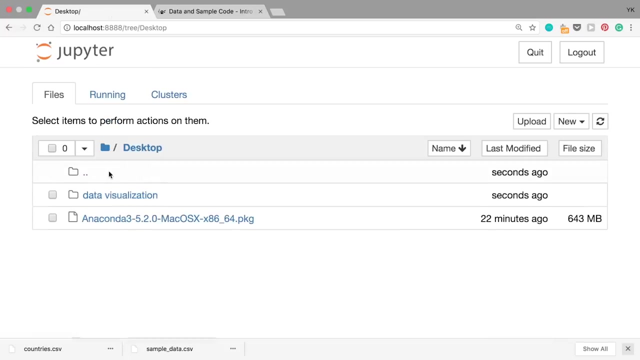 So let's first download our data. To do that, just go to csdojoio slash data and download these two files- sample data, csv and countriescsv- and then put these csv files in the folder that you just created: Data visualization. After that, go back to the Jupyter Notebook interface and you can just navigate to desktop. 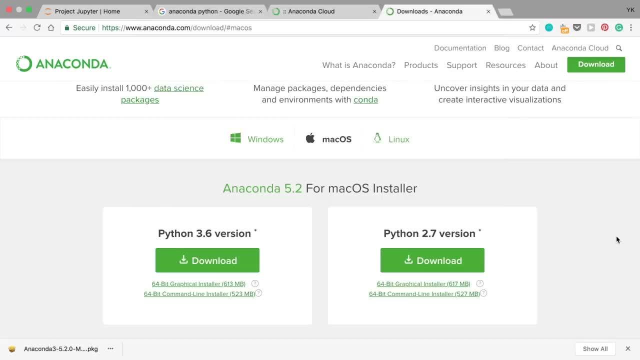 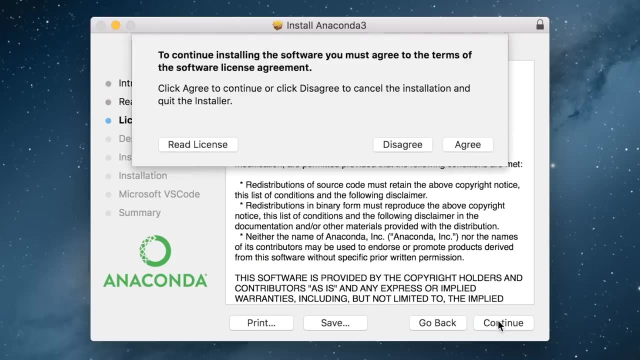 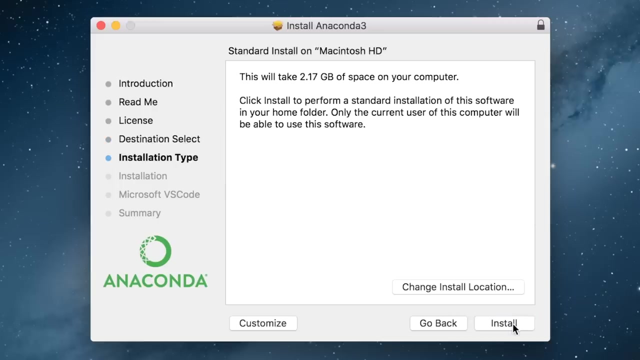 download this package, save it And, once it's downloaded, open up the package that you just downloaded and then just click continue, continue, continue, continue, Agree. install for me only or install on a specific disk, It doesn't matter which one- and continue and click install. 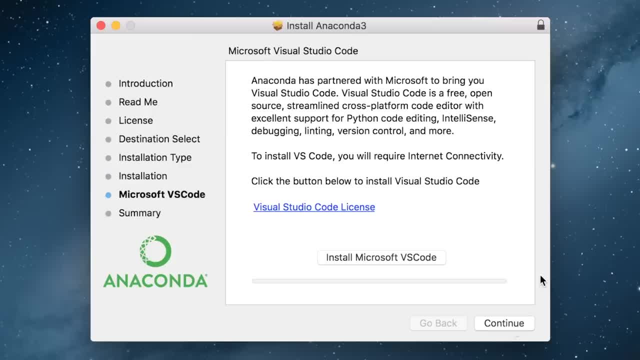 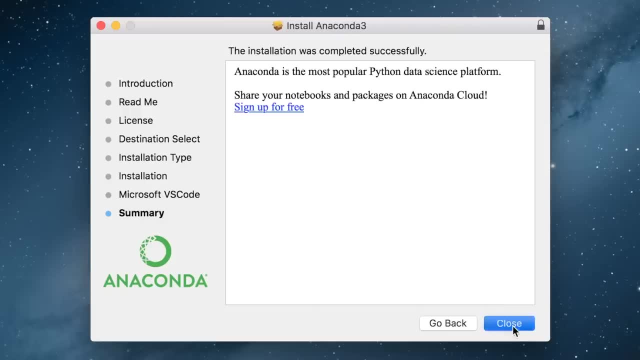 And this process is going to take a while. After some waiting, you might see this prompt to install Microsoft VS code. We don't need that, So let's just continue here and then close. And then to launch Jupyter Notebook. you can do it through this thing called Anaconda Navigator. 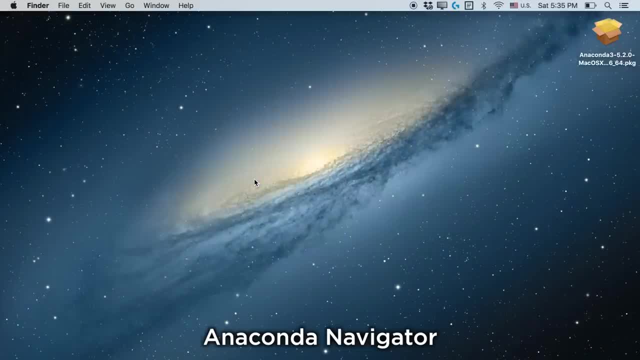 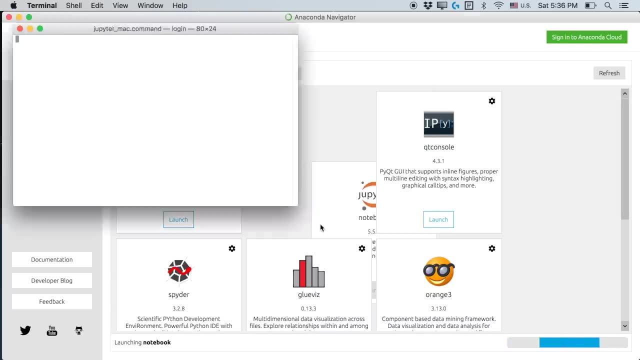 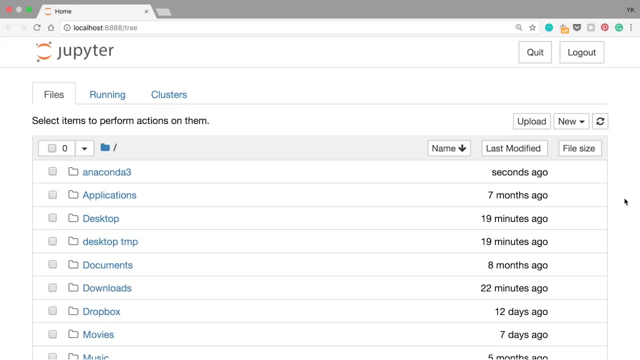 So just launch it like you launch any other application: Just dismiss whatever comes up and then click launch in the Jupyter Notebook section, And then you should see a browser window show up with the Jupyter Notebook interface. Now, if you want to follow this tutorial, the first thing you should do is you should create a new. 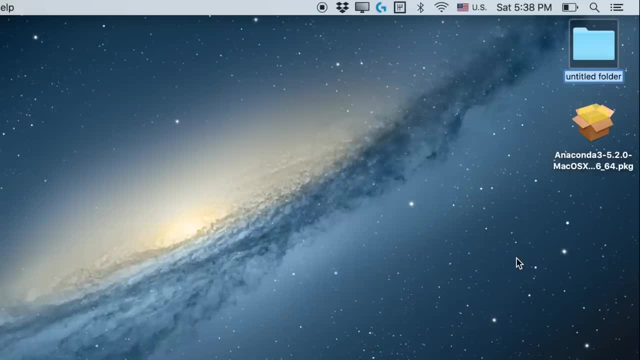 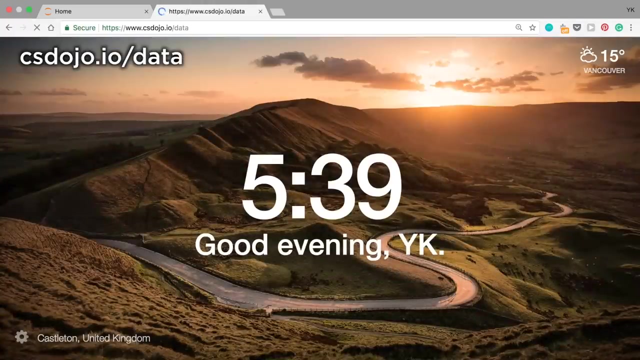 folder, let's say on desktop, And let's call this one data visualization, And we're going to put all our data and Jupyter Notebook file here. So let's first Download our data. to do that, Just go to CS, dojoio, slash data and download these two files. sample data: CSV and countries that. 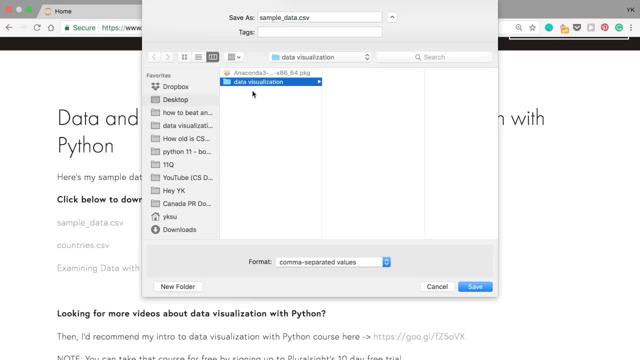 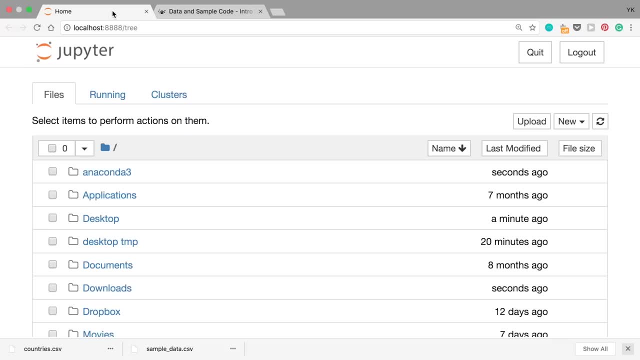 CSV and then put these CSV files in the folder that you just created- data visualization. After that go back to the Jupyter Notebook interface and you can just navigate to desktop and then the folder that we just created- data visualization- and to create a new Jupyter Notebook. 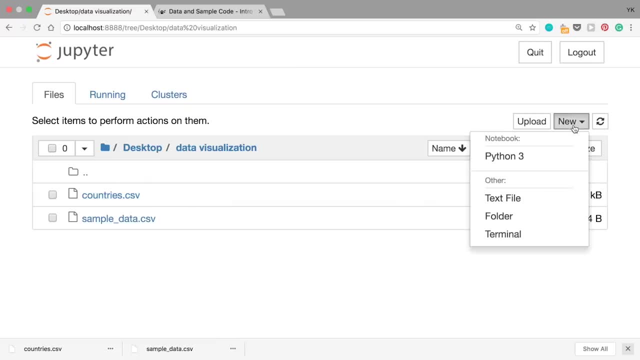 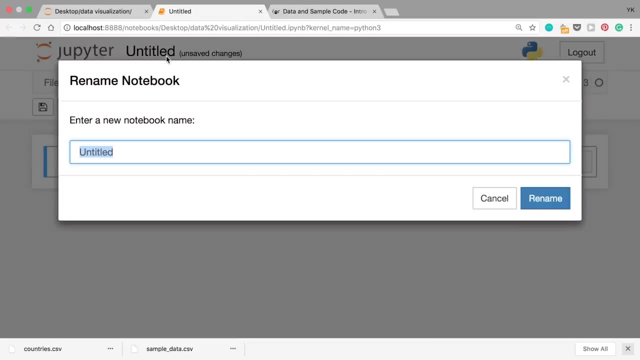 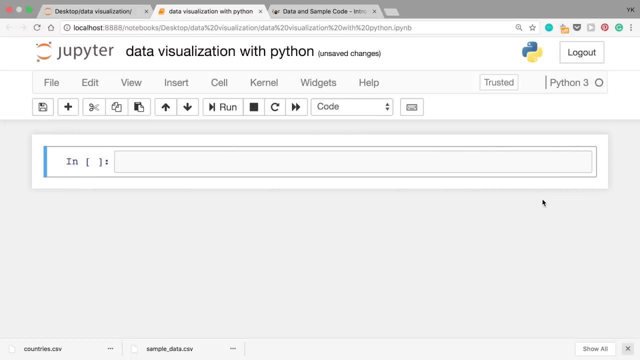 file Here. just find the new button on the right and click Python three. Right now this notebook file has untitled as the title, So let's change it to data visualization with Python. Click rename and you have a notebook called data visualization with Python. 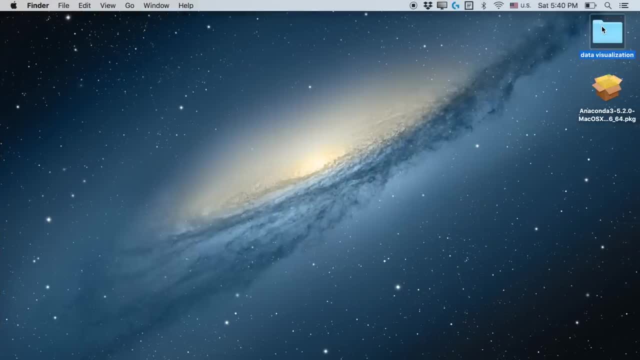 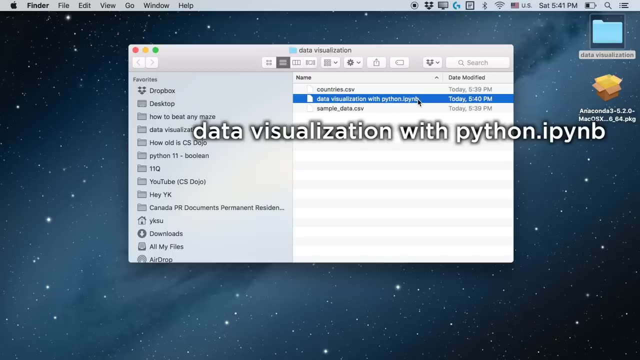 You can check it just by going to desktop and then to the folder that you just created, And you should see that there's a file called data visualization with Python, And it's really important that this notebook file is in the same folder as the data that. 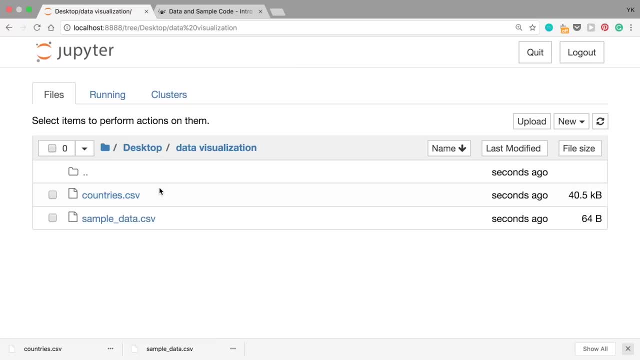 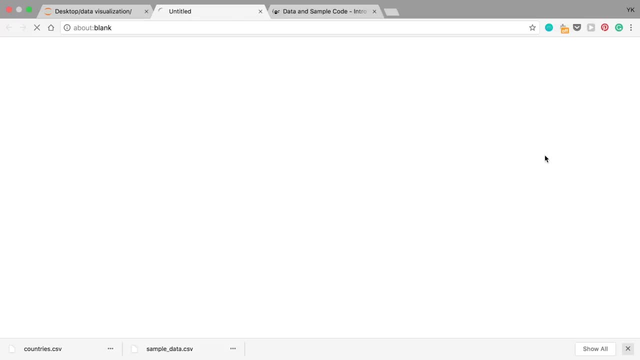 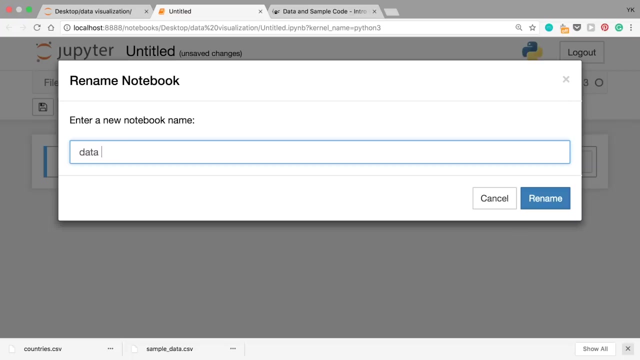 and then the folder that we just created, Data visualization. And to create a new Jupyter Notebook file here, just find the new button on the right and click Python three. Right now, this notebook file has untitled as the title, So let's change it to data visualization with Python. 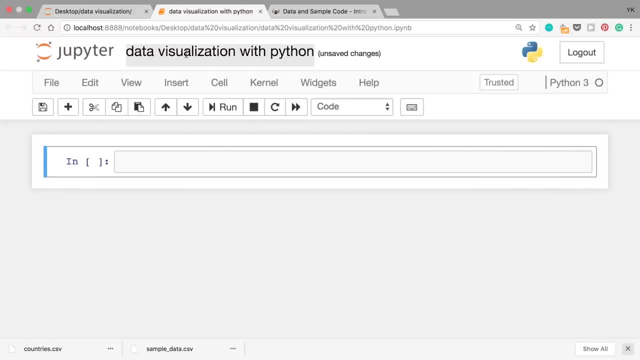 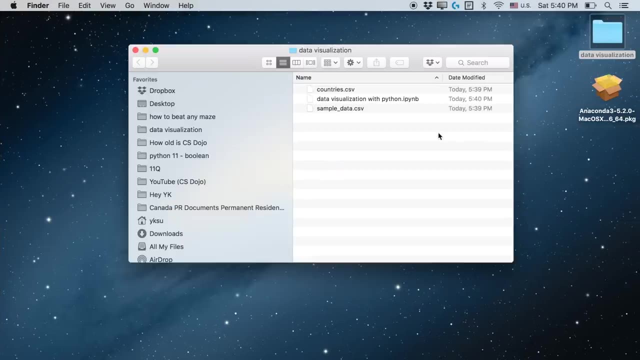 Click rename and you have a notebook called data visualization with Python. You can check it just by going to desktop and then to the folder that you just created, And you should see that. Okay, So let's go back. There's a file called data visualization with pythonipynb. 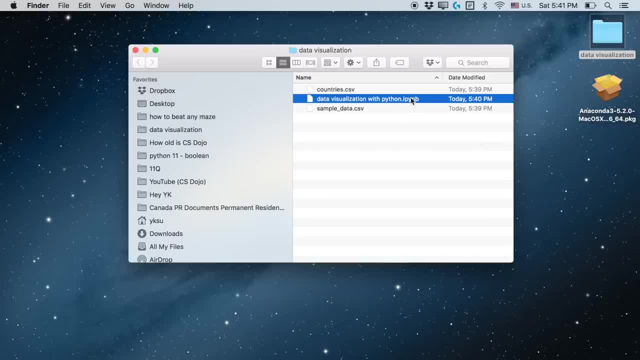 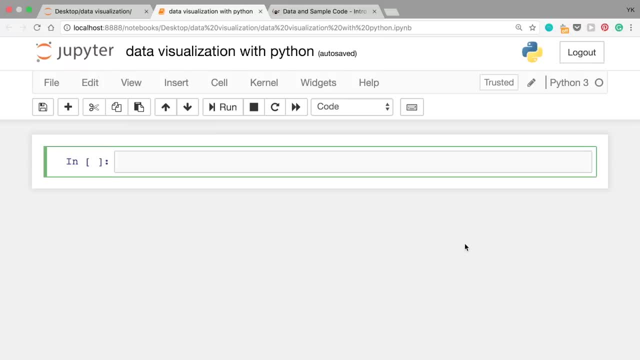 And it's really important that this notebook file is in the same folder as the data that you just downloaded- countriescsv and the other one- And once everything is set up, just write in the first cell: import pandas as pd. This means we want to import a module called pandas as pd or we want to give it sort of 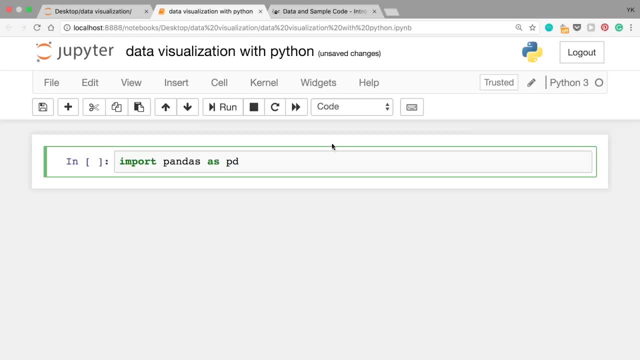 a nickname And that's going to be pd. You can run this cell by clicking this button And now pandas is imported as pd, And here we're going to use pandas for importing and using some data from our csv files And we need to import another module here. 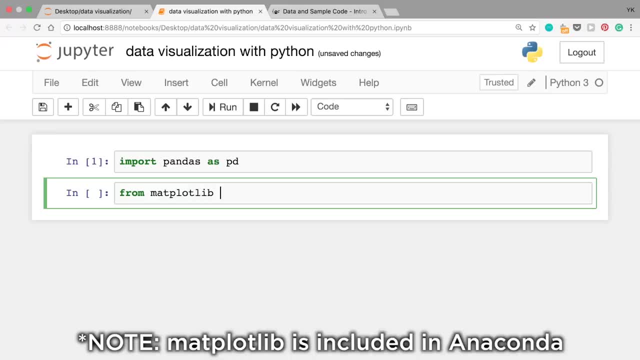 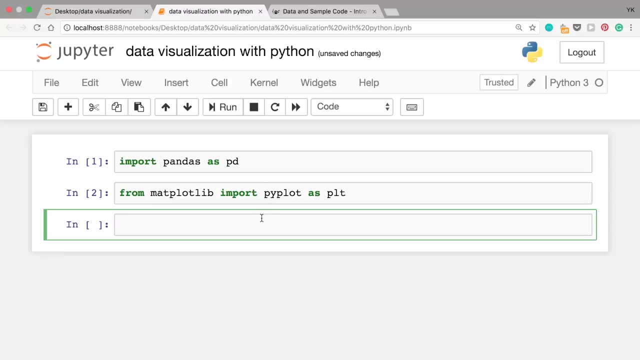 So for that just write: from matplotlib, import pyplot as plt. So this says: from the matplotlib package, import pyplot module and then call it plt And that's going to be pd. Okay, Let's run this cell, And now pyplot is imported. 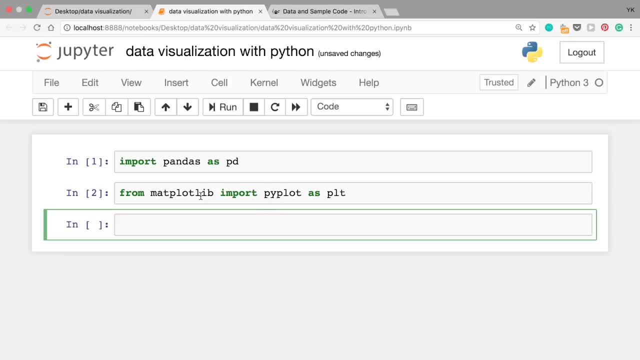 We're going to use pyplot from matplotlib for making our charts. So here let's first take a look at a really simple example of how to use pyplot. So here I'm going to write: x equals one, two, three. It's a list of three elements. 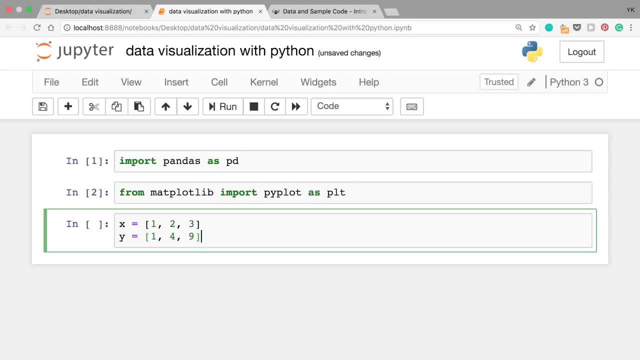 And y equals one, four and nine, And to plot this set of data you can just write pltplot And this plots x on the x-axis and y on the y-axis. You can show this graph by writing pltshow. When you run the cell you should see a graph like this: 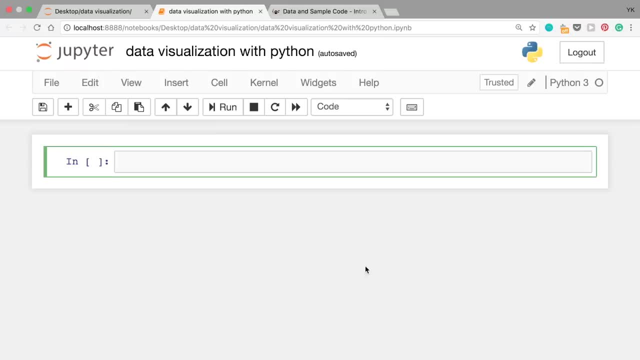 you just downloaded countries, that CSV and the other one, And once everything is set up, just write in the first cell: import pandas as PD. This means we want to import a module called pandas as PD or we want to give it sort of. 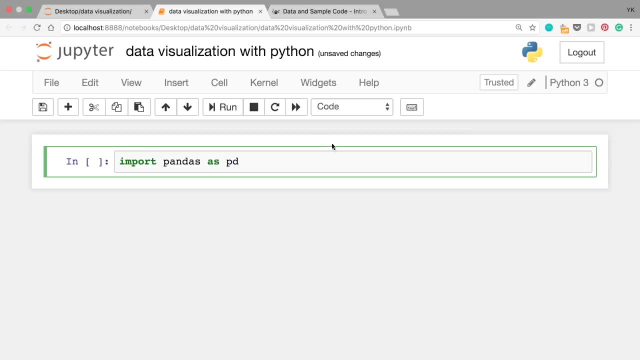 a nickname and that's going to be PD. You can run the cell by clicking This button and now pandas is imported as PD, And here we're going to use pandas for importing and using some data from our CSV files And we need to import another module here. 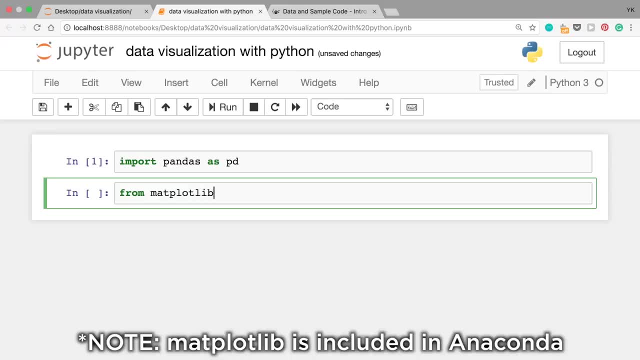 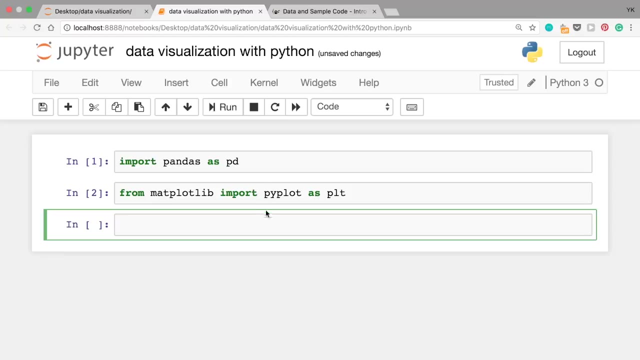 So for that just write: from matplotlib import PyPlot as PLT. So this says: from the matplotlib package import PyPlot module and then call it PLT. Let's run this cell And now PyPlot Is imported. We're going to use PyPlot from matplotlib for making our charts. 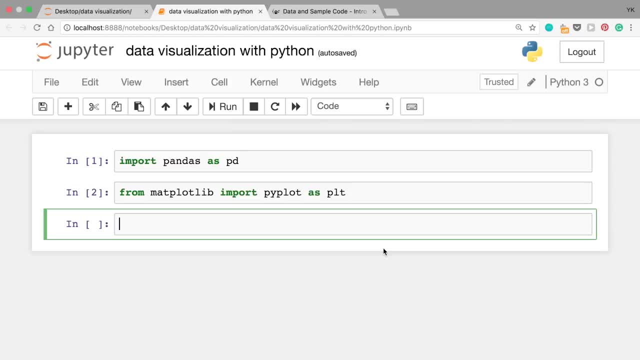 So here let's first take a look at a really simple example of how to use PyPlot. So here I'm going to write: X equals one, two, three- It's a list of three elements- and Y equals one, four and nine. 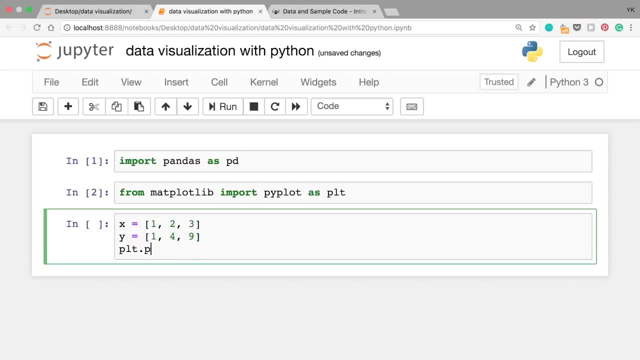 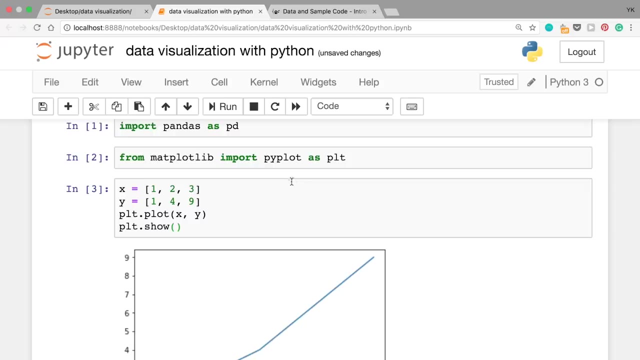 And to plot this set of data you can just write PLT dot plot X, comma Y, and this plots X on the X axis And Y on the Y axis. And then you can show this graph by writing PLT dot show. And when you run the cell you should see a graph like this: 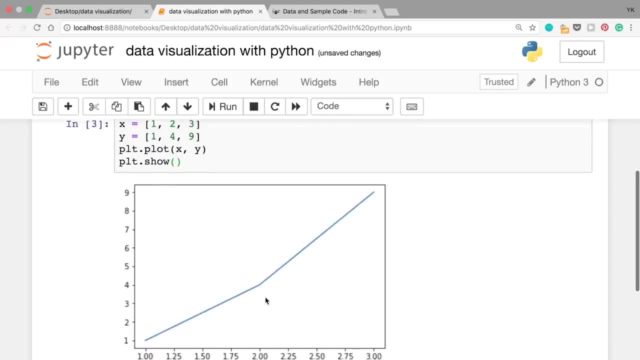 You see that the values of X are one, two and three, as expected, And the values of Y are one, four and nine. If you want to add a title to this graph, you can do so by writing PLT dot- title tests plot right after the plot statement. 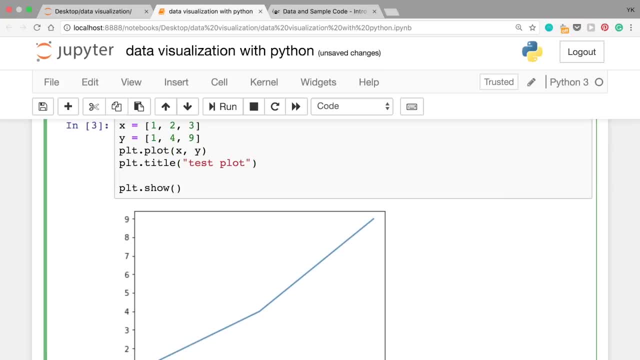 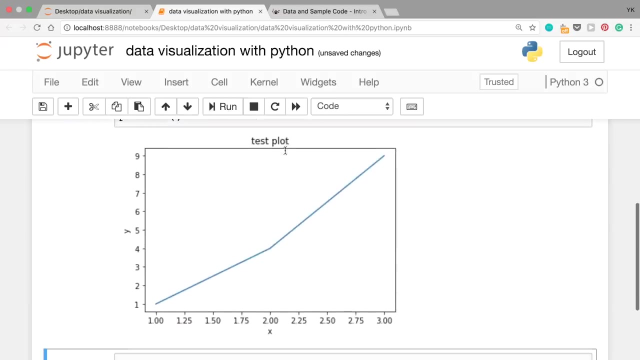 before the show statement. and then you can add an x label and the y label as well by writing: pltx label, let's call the x label x, and plty label, let's call the y label y here. and when you run this cell, you'll see that there's a title called test plot and x label called x and y label called 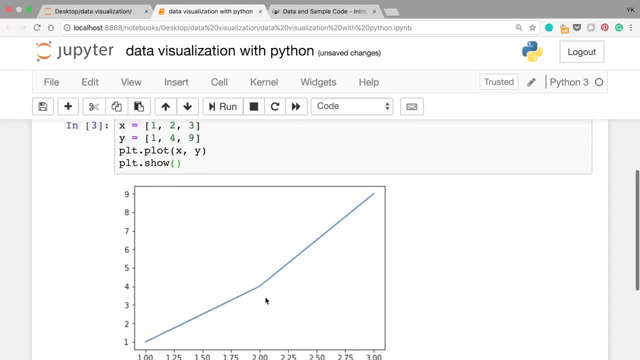 You see that the values of x are one, two and three, as expected, And the values of y are one, four and nine. If you want to add a title to this graph, you can do so by writing plttitletesplot". 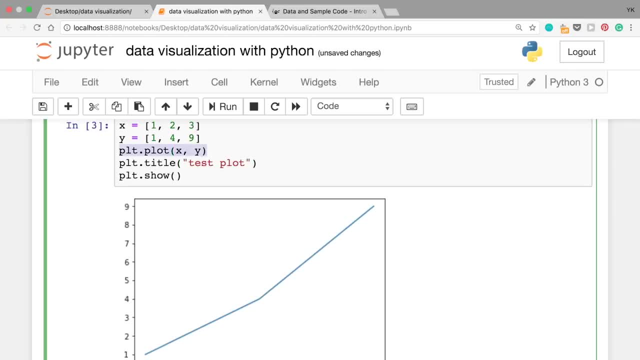 d-ray: y-axiscom plot, right after the plot statement, before the show statement, and then you can add an x label and the y label as well by writing: plt dot x label- let's call the x label x, and plt dot y label- let's call the y label y here. and when you run this cell you'll see that there's a title called 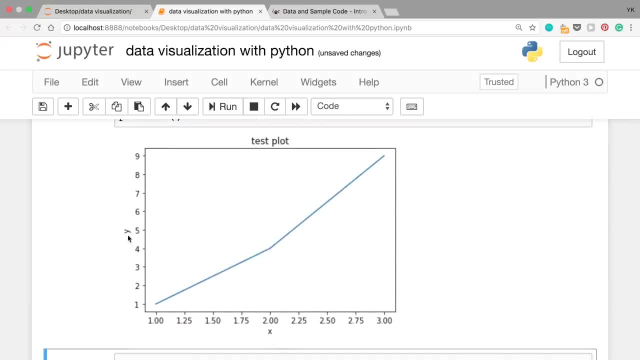 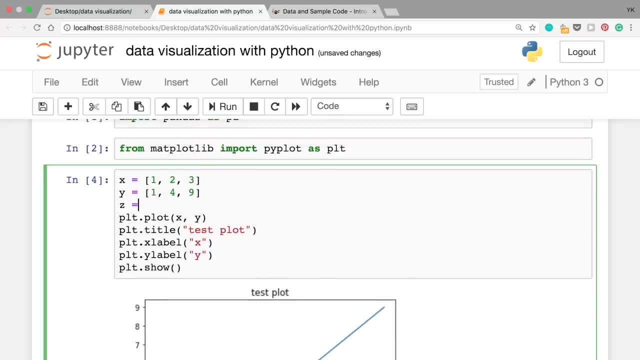 test plot and x label called x and y label called y. okay, what if you wanted to plot multiple lines here? well, to do that, let's create another list. let's call it z, and this one is going to have 10, 5 and 0 inside. and to plot x and z on top of x and y, you can just write plt, dot, plot x, comma z. 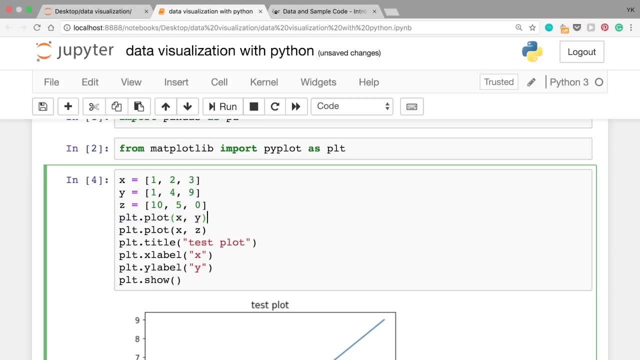 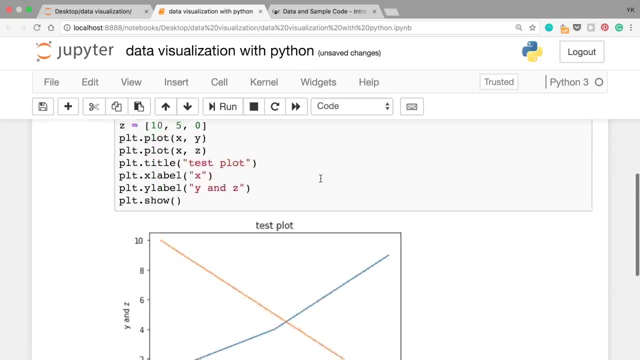 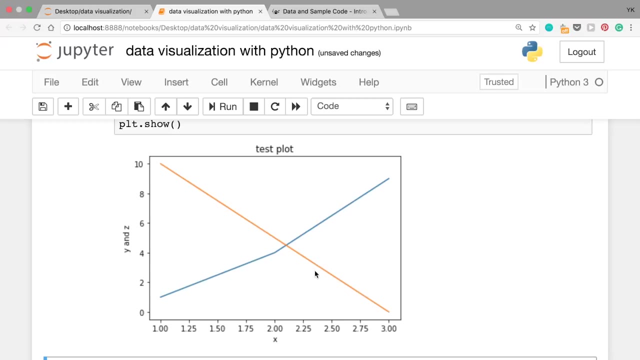 right after plt, dot, plot x, comma y, and then let's fix the y label here to y and z, and when you run this cell you should see, you should see, you should see these two lines. so the blue line represents x and y and the orange line represents x and z. 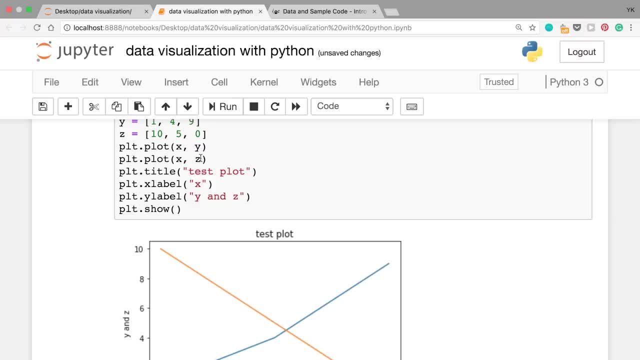 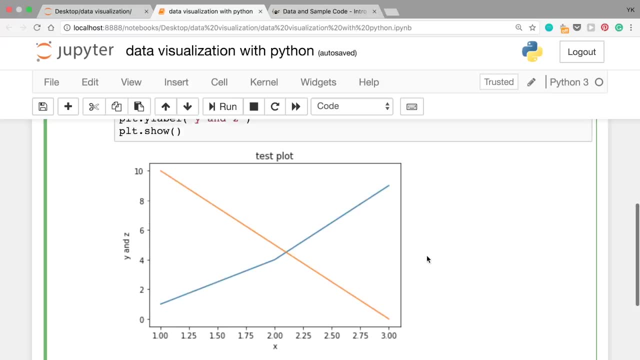 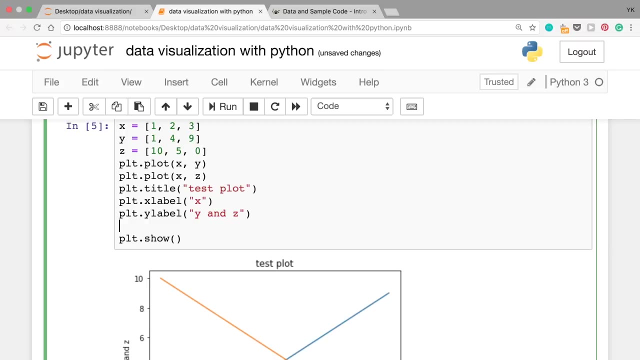 so plt dot plot x and z. plot it: x on the x-axis and z on the y-axis. but right now it's kind of hard to tell which line represents which data. so we can fix it by adding a legend statement. let's add that after the y label statement by writing plt dot legend, parentheses, square brackets. 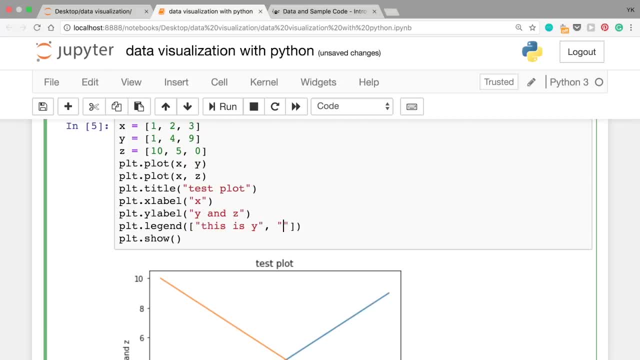 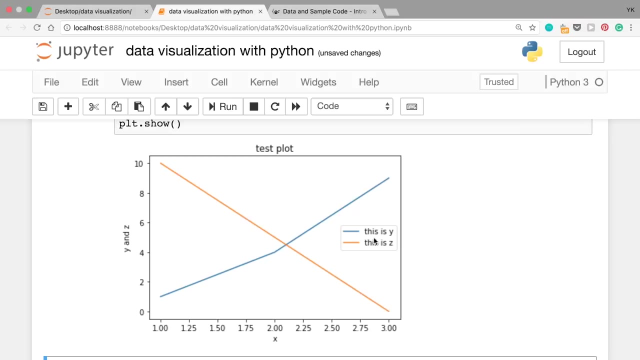 double quotes: this is y. comma. double quotes: this is z. so note here that this legend function takes a list as an argument, and when you run this cell you should see this legend that says: the blue line is this is y and the orange line is this is z. okay, that's the basics of plotting. now let's see. 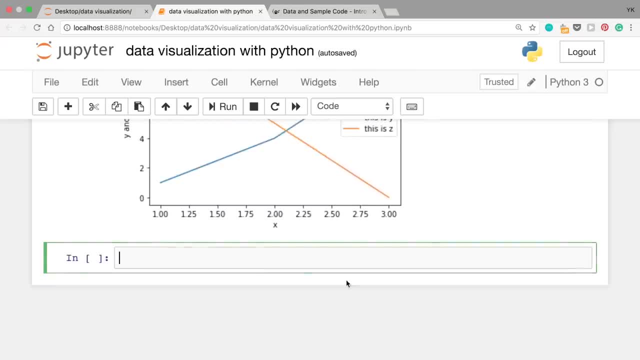 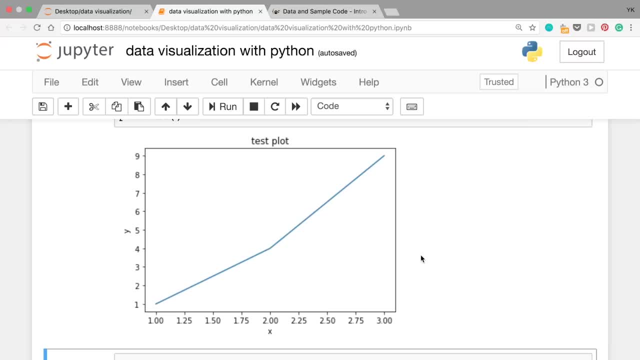 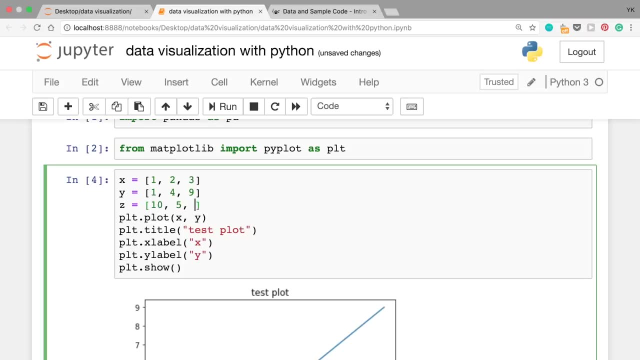 y. okay, what if you wanted to plot multiple lines here? well, to do that, let's create another list. let's call it z, and this one is going to have 10, 5 and 0 inside, and to plot x and z on top of x and y. 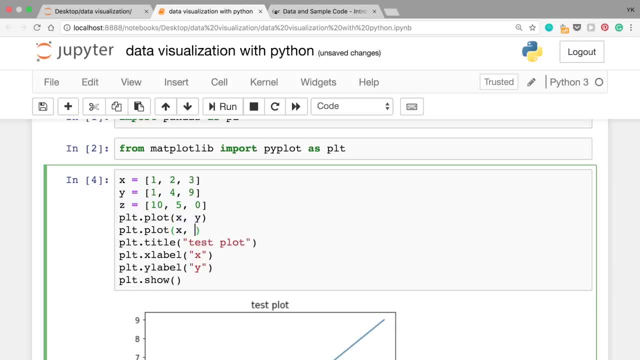 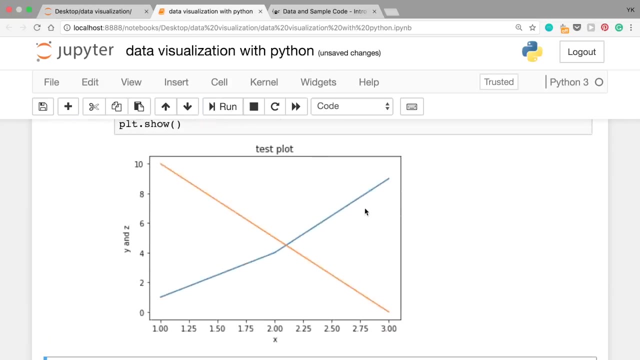 you can just write plt dot plots x, comma z right after plt dot plot x, comma y, and then let's fix the y label here to y and z, and when you run this cell you should see these two lines. so the blue line represents x and z. 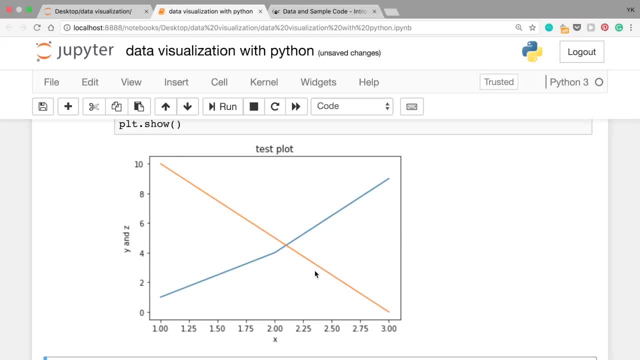 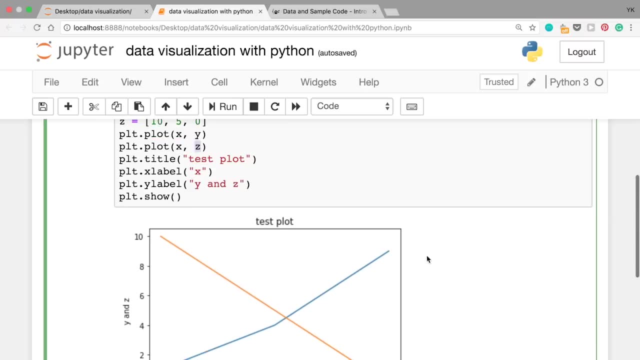 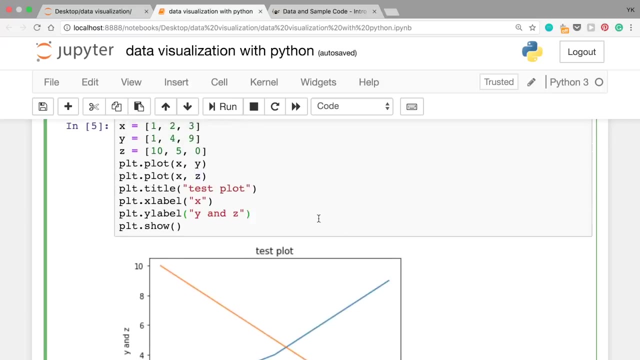 y and the orange line represents x and z. so plt dot. plot x and z. plot it: x on the x-axis and z on the y-axis. but right now it's kind of hard to tell which line represents which data. so we can fix it by adding a legend statement. let's add that after the y level statement by writing plt dot. 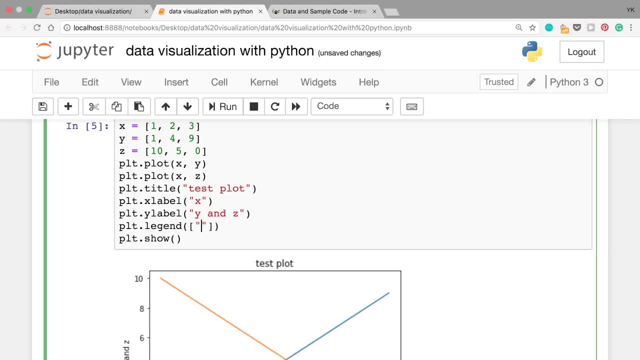 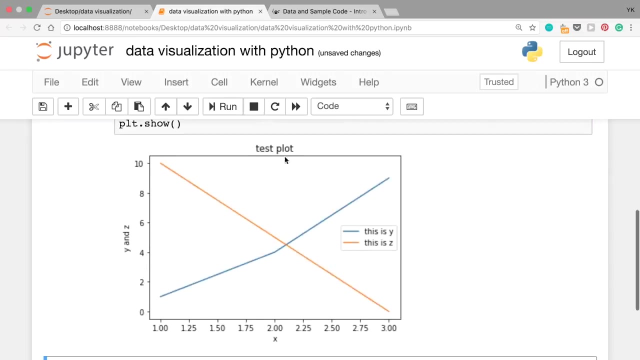 legend: parentheses, square brackets. double quotes: this is y. comma. double quotes: this is z. so note here that this legend function takes a list as an argument and when you run this cell you should see this legend that says: the blue line is: this is y and the orange line is: this is z. okay, that's. 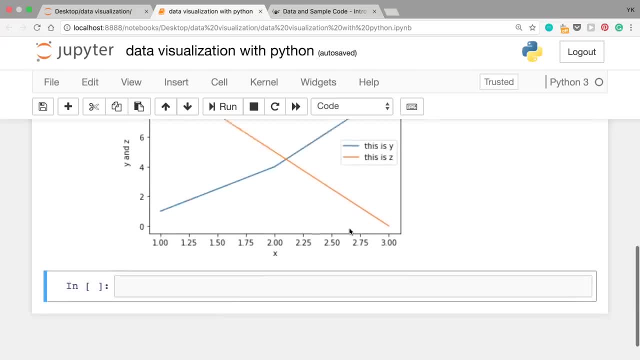 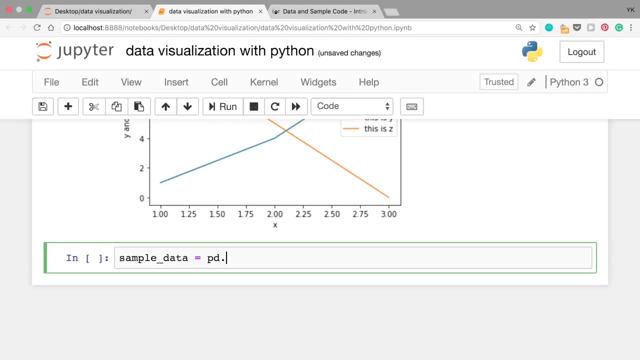 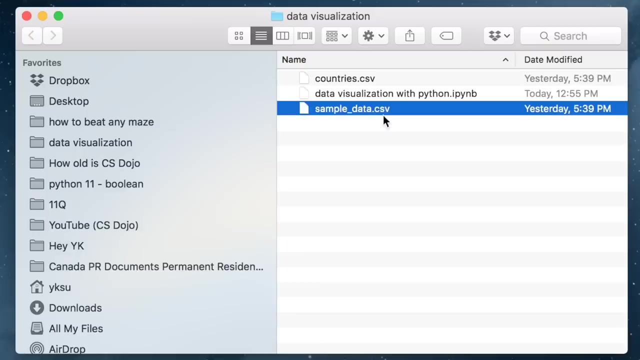 the basics of plotting. now let's see how to load data from a csv file. for that you can just write: sample underscore data equals pd or pandas dot read csv. by the way, i just pressed tab here to do autocomplete and then parentheses: sample underscore data dot csv. now, before you run this cell, make sure that the notebook file data. 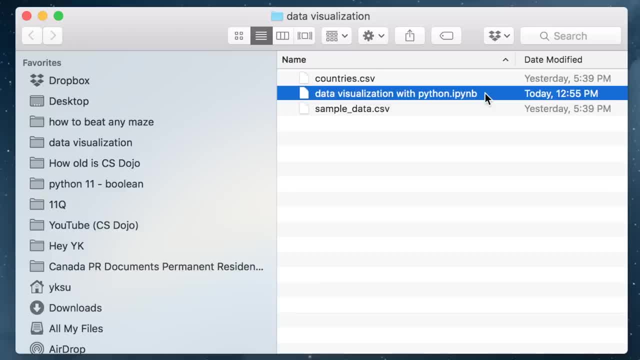 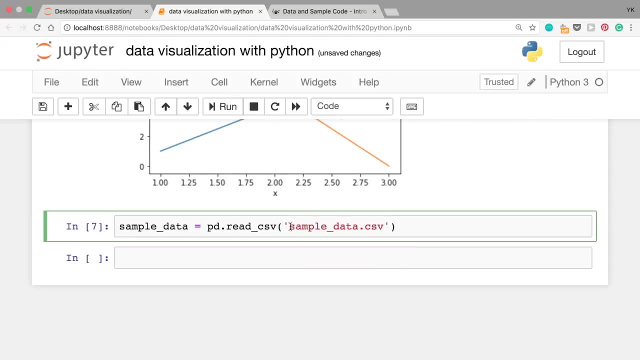 visualization with pythonipy nb is in the same folder as sampledatacsv. when you run the cell, this data, sample datacsv. when you run this cell, this data, sample data- that csv is loaded by the pandas module, which we call pd, and then it's assigned to this variable. 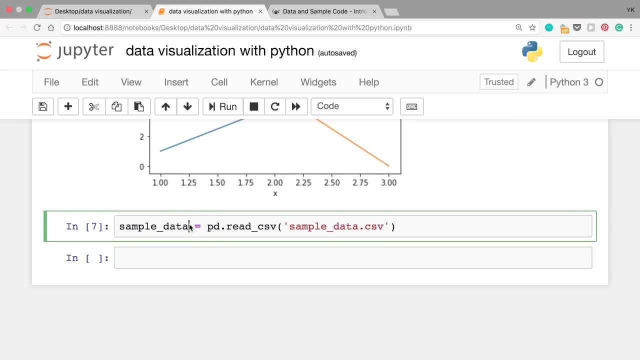 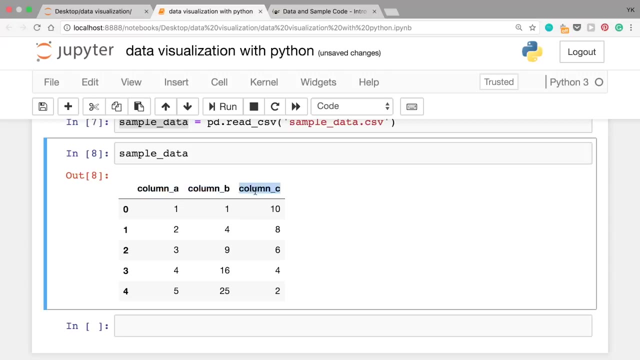 called sample data. you can check what's inside this variable sample underscore data just by writing sample underscore data in this new cell and then, when you run this cell, you should see something like this: so, as you can see, this data has three columns: column a, column b and column c. 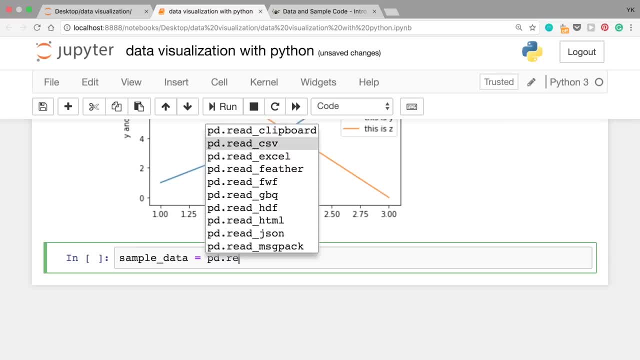 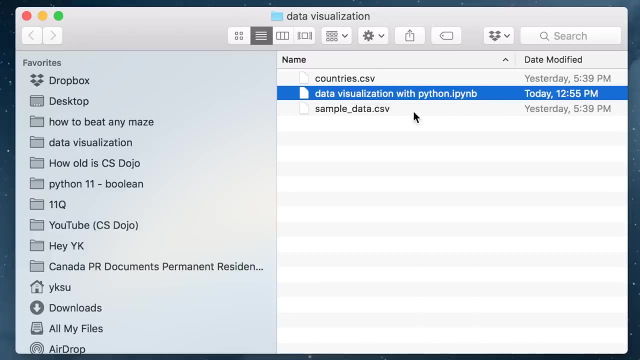 equal to pd or pandas dot read csv. by the way, i just press tab here to do auto complete and then, uppermost parentheses, sample underscore data dot csv. now, before you run this cell, make sure that the notebook file data visualization with python dot ipy and b is in the same folder as sample data. 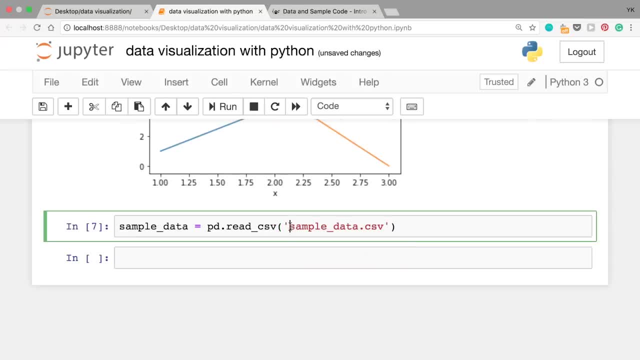 dot csv. when you run this cell, this data- sample data, dot csv- is loaded by the pandas modules and which we call pd, and then it's assigned to this variable called sample data. you can check what's inside this variable- sample underscore data- just by writing sample underscore data in this new 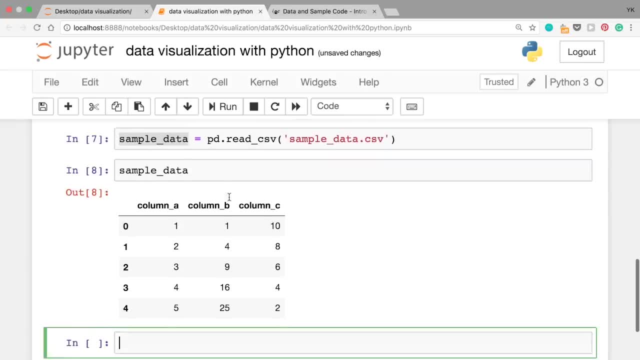 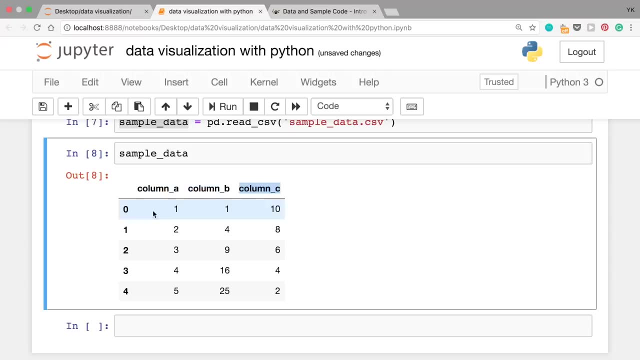 cell and then when you run this cell, you should see something like this: so, as you can see, this data has three columns- column a, column b and column c- and five rows, and you see a bunch of values inside this table. if you want to check if this set of data is exactly the same as the 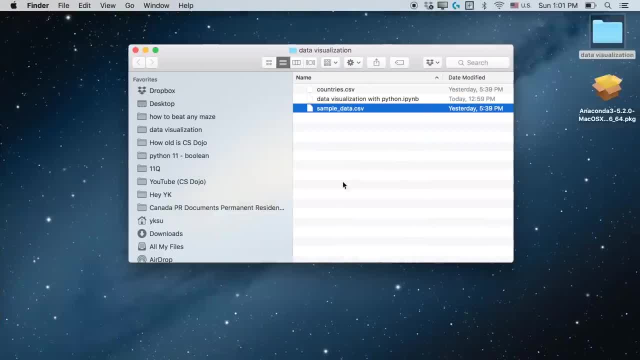 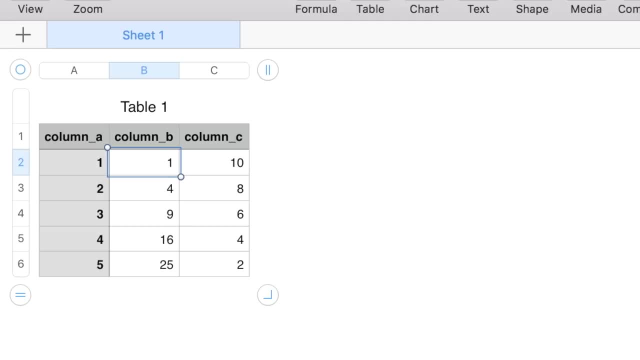 original data. you can do so by opening up the original data file- sample data, dot csv- with excel or any other spreadsheet application, and when you open it you should see exactly the same data: column a, column b, column c, with five rows with a bunch of values. okay, the only difference that 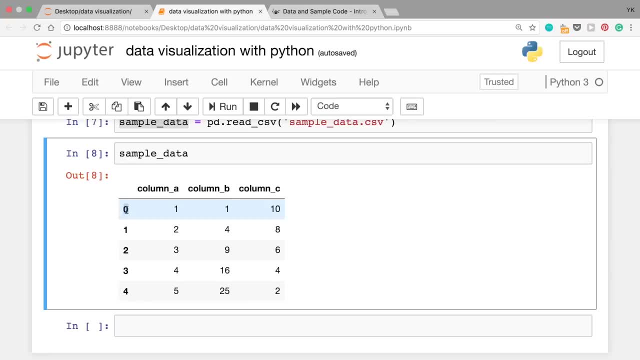 you might see is that in jupyter notebook you might see these numbers zero, one, Green, R and yellow maker or like flam. Nacional. the number one row is actually going to go to two, three and four, and these are just indices for the rows and you can check what type this variable. 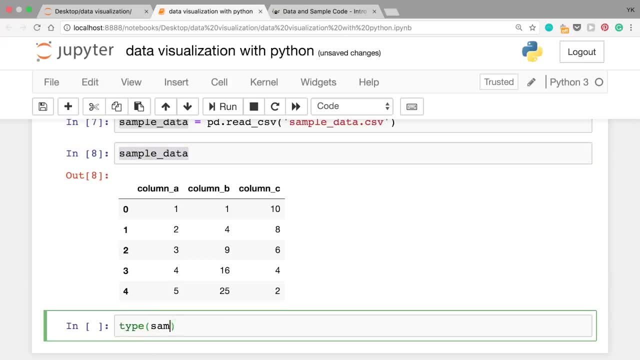 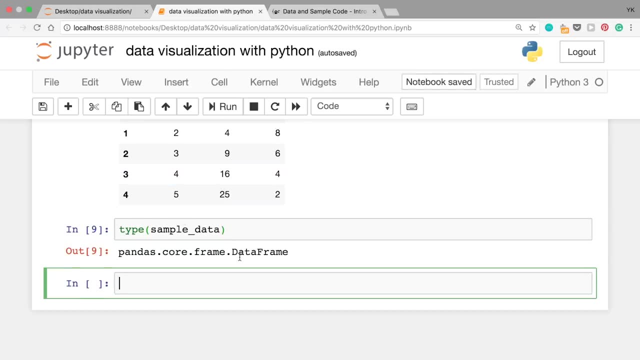 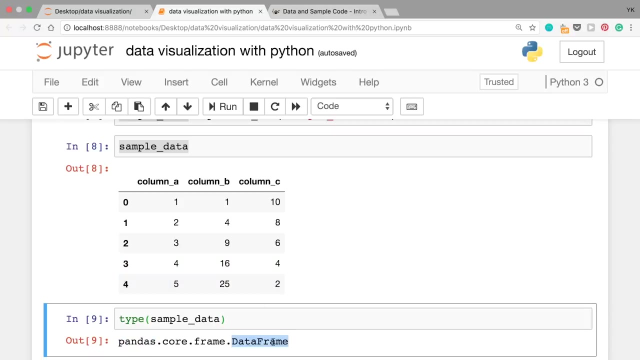 is by writing type parentheses, sample underscore data and when you run this cell it says that this is pandascoreframedataframe. so this is a data frame type that's defined by the pandas module and the data frame type is used to contain a table like piece of information, just like this one. okay, 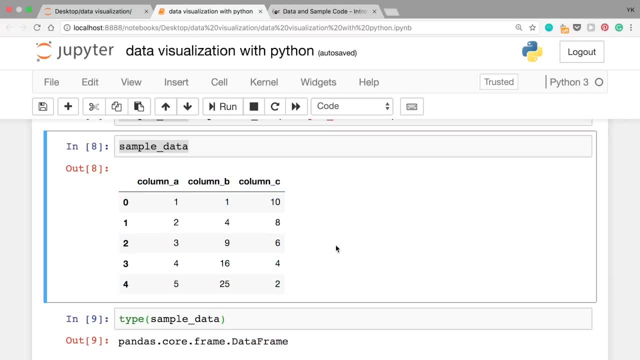 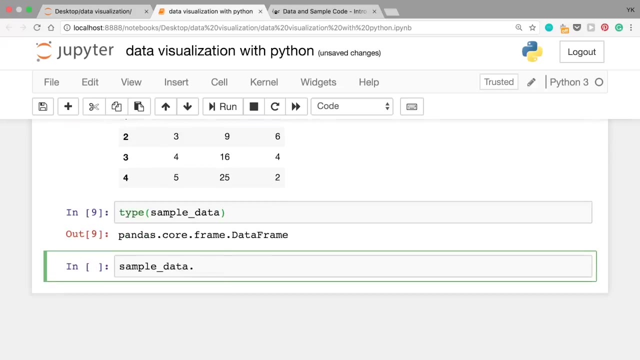 now what if you wanted to plot data in this data frame, for example the values of column a on the x axis and column c on the y axis? well, to do that, you'll need to be able to retrieve a specific column, and you can do that by writing sample underscore data: dot column, dot. c column- underscore. 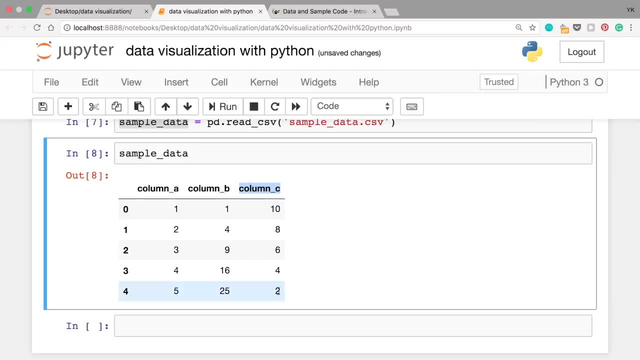 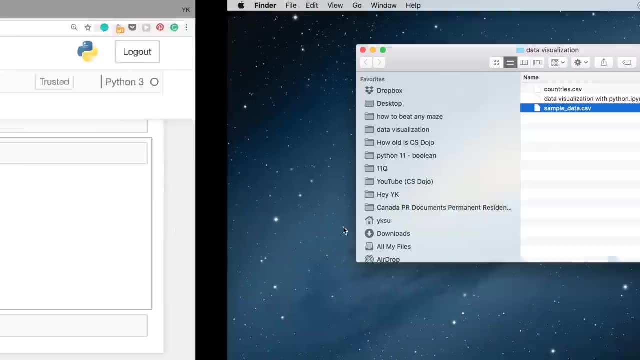 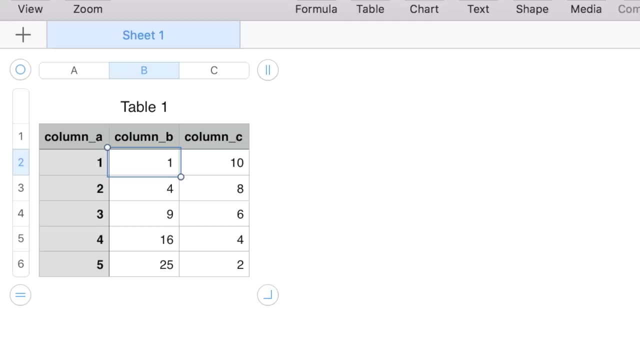 and five rows and you see a bunch of values inside this table. if you want to check if this set of data is exactly the same as the original data, you can do so by opening up the original data file- sample, datacsv- with excel or any other spreadsheet application, and when you open it, you 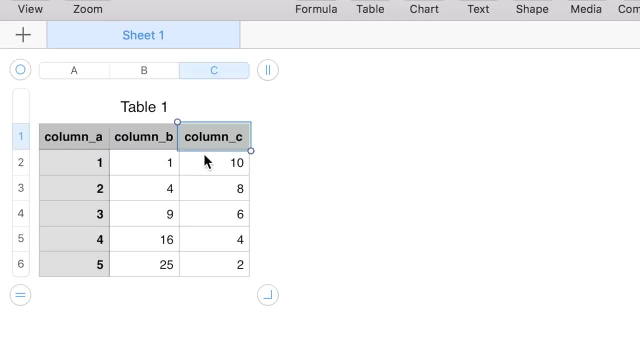 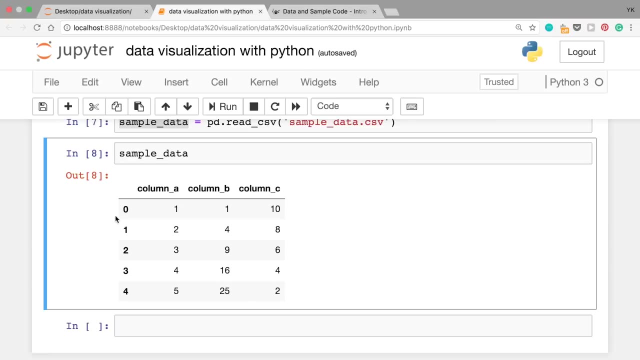 should see exactly the same data- column a, column b, column c- with five rows with a bunch of values. okay, the only difference that you might see is that in jupyter notebook you might see these numbers 0, 1, 2, 3 and 4, and these are just indices for the rows, and you can. 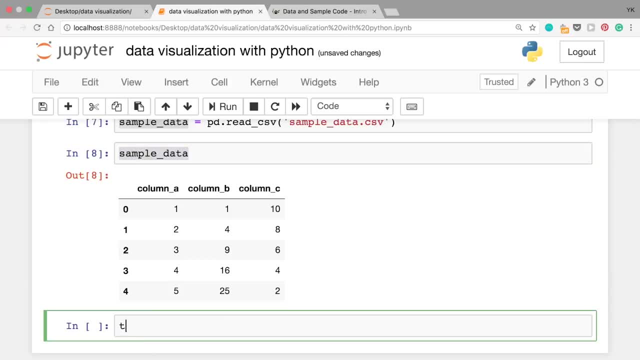 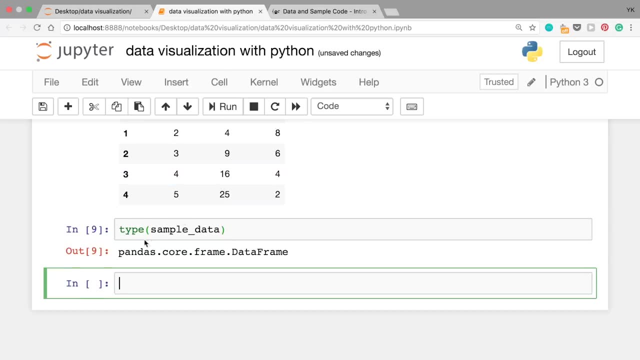 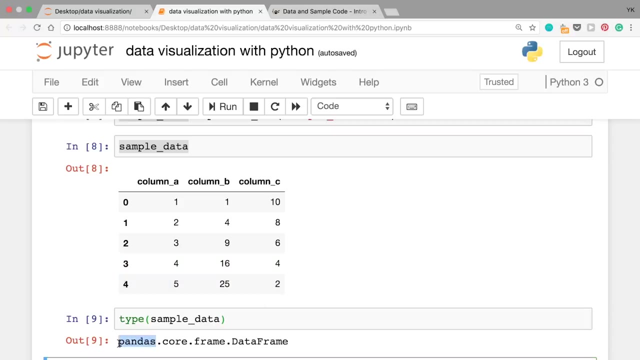 check what type this variable is by writing type, parentheses, sample, underscore data and when you run this cell, it says that this is pandascoreframedataframe. so this is a data frame type that's defined by the pandas module, and the data frame type is used to contain a table-like piece. 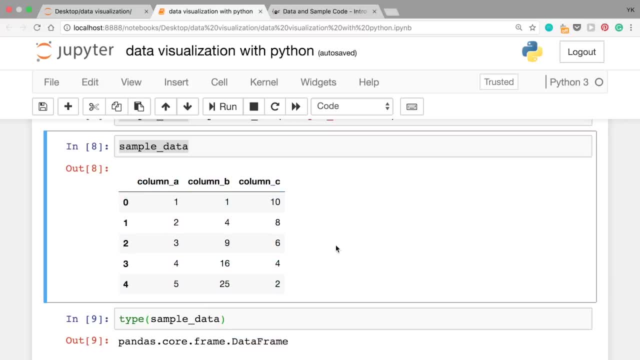 of information for the data that you want to use when you run this cell and then you can see that just like this one. okay, now what if you wanted to plot data in this data frame, for example, the values of column a on the x-axis and column C on the y-axis? 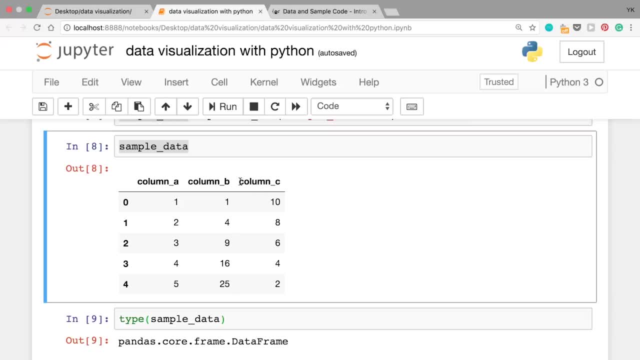 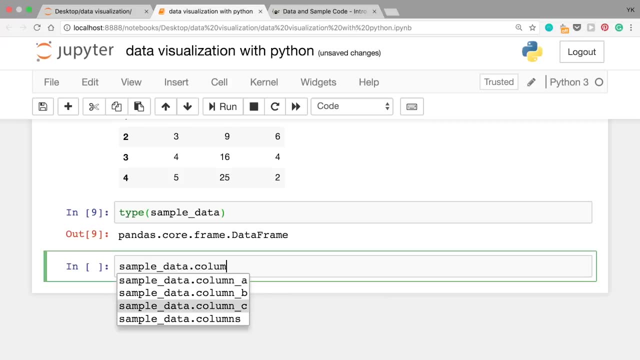 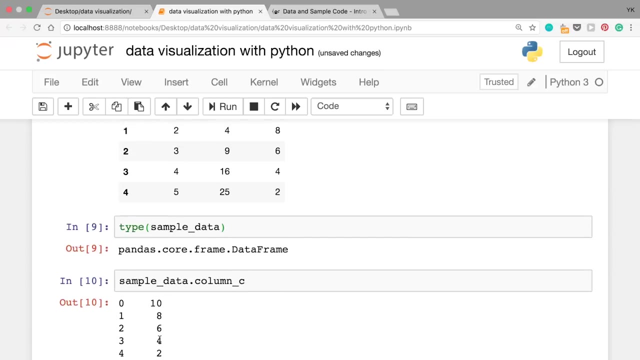 well, to do that, you'll need to be able to retrieve a specific column and you can do that by writing sample underscore data: dot. column, dot C. column underscore C. when you run this cell, you'll see that the column C is retrieved. it has the values 10, 8, 6, 4 and 2, and the numbers you see on the left are just indices: 0- 1. 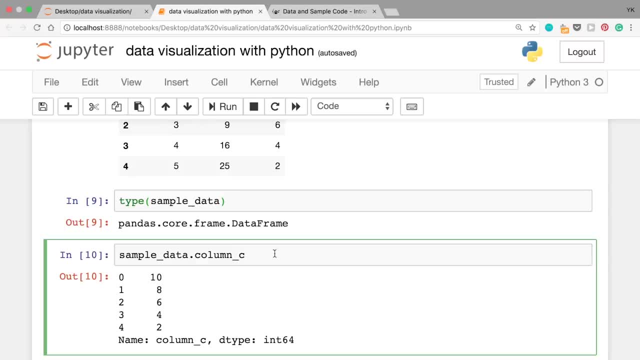 2, 3 and 4, just like before. you can check what type this is by writing type parentheses: sample data: dot, column C. and when you run this cell you see that this is pandas, dot core, dot series, dot series. so this is basically a series type. 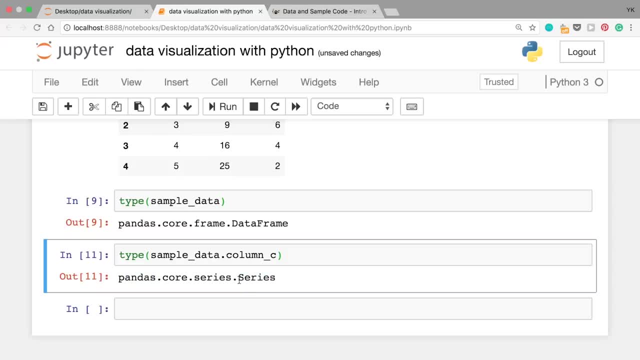 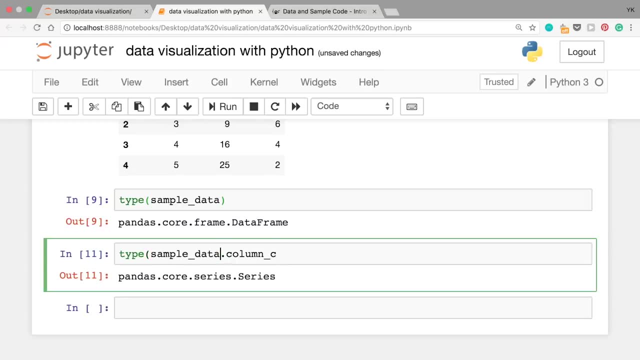 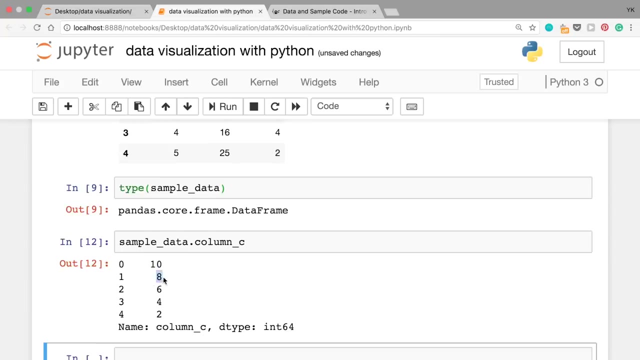 that's defined by the pandas module and it's a type that's used to store a series of values, for example, these values: 10, 8, 6, 4 and 2. now, what if you wanted to retrieve a specific value out of this series? well, if you want to retrieve, for example, the second value here, 8, you can. 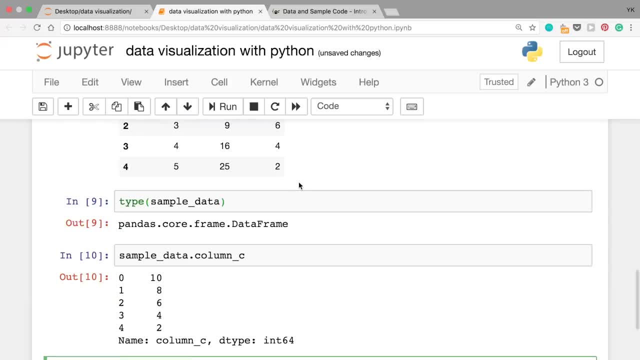 c. when you run this cell, you'll see that the column c is retrieved. it has the values 10, 8, 6, 4 and 2, and the numbers you see on the left are just indices: 0, 1, 2, 3 and 4.. just like before, you can check what type this is by writing type. 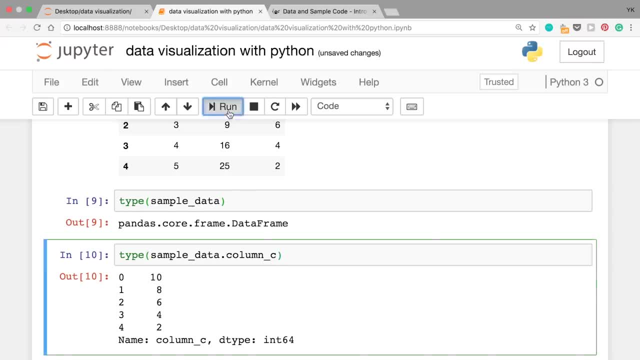 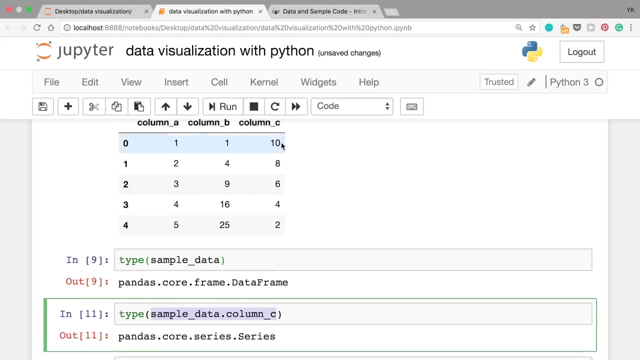 parentheses: sample data: dot column c. and when you run this cell you see that this is pandascore seriesseries. so this is basically a series type that's defined by the pandas module and it's a type that's used to store a series of values. for example, these values: 10, 8, 6, 4 and 2.. 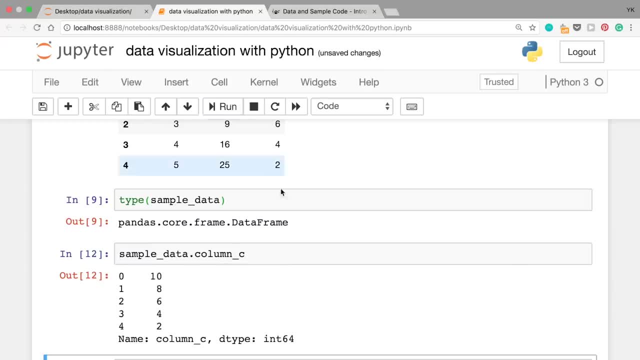 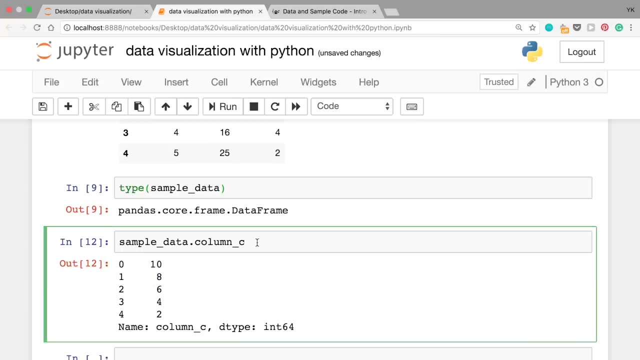 now, what if we wanted to retrieve a specific value out of this series? well, if you want to retrieve, for example, the second value here, 8, you can do so by writing sample data: dot, column c, dot i, loc i, l, o, c, square brackets 1, and this retrieves the second value of. 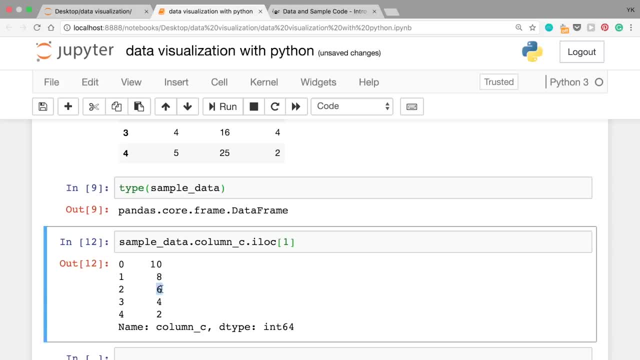 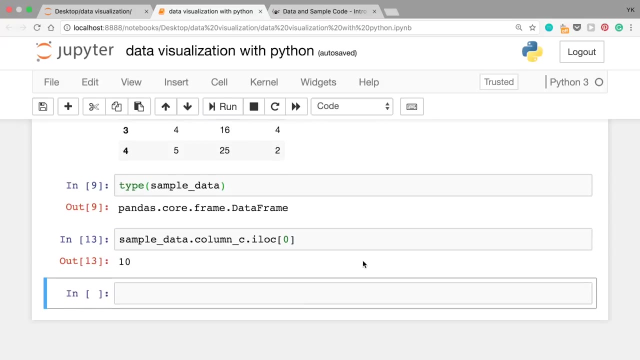 the series 8, and if you want to retrieve the third value, 6, you can write i loc 2, and that gets the third value. and if you want to retrieve the first value, you can write i loc 0, and this should give us the third value of the series and it does. okay, and using what we've just learned here, we'll be able. 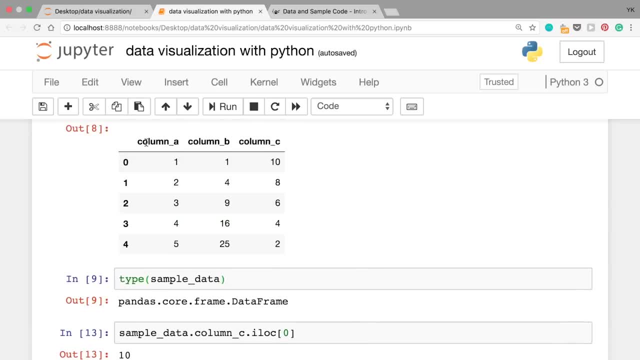 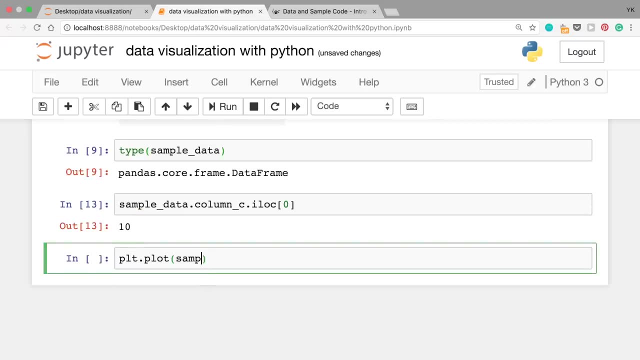 to plot the data in this data frame. so let's say we want to plot column a on the x-axis and column b on the y-axis. we can do that by writing pltplots: sample data dot- column a. comma. sample data dot- column b. and we can show it by writing pltshow. let's see how it looks. we have one, two, three. 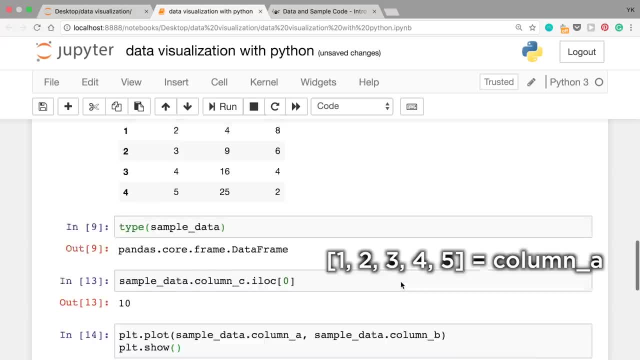 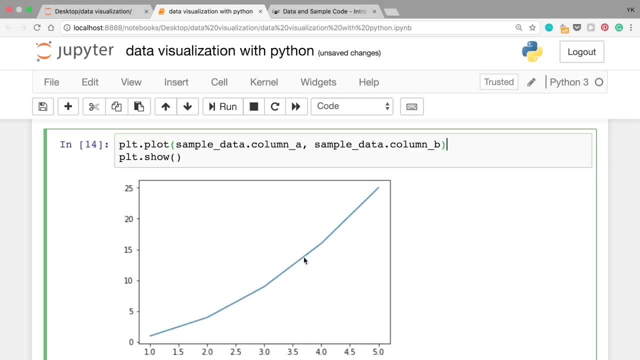 four and five on the x-axis and on the y-axis we have one, four, nine, 16 and 25, as expected. if you want to add column c to this data, you can write pltplots: sample data dot column a. so let's use column a as the x-axis again and sample data dot column c. when you run the cell you see that there. 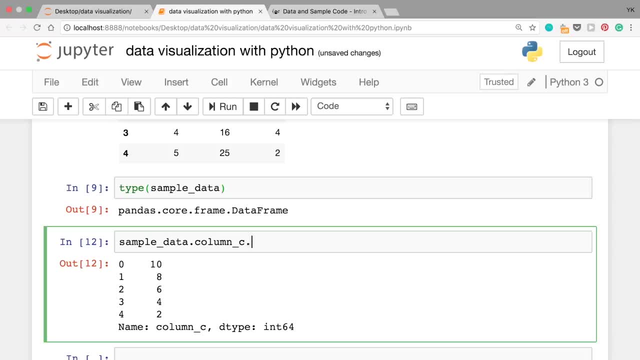 do so by writing sample data: dot, column C, dot iloc, square brackets 1, and this retrieves the second value of the series 8. and if you want to retrieve the third value, 6, you can write iloc 2, and that gets the third value. and if you want to, 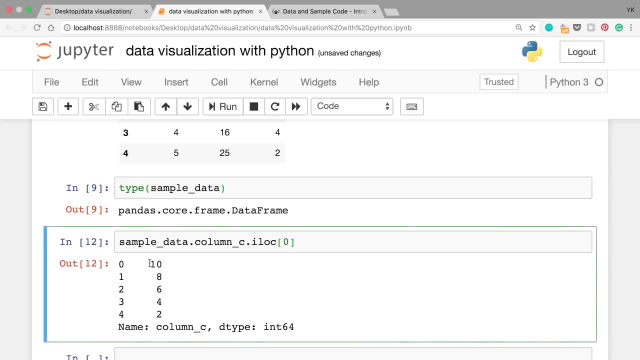 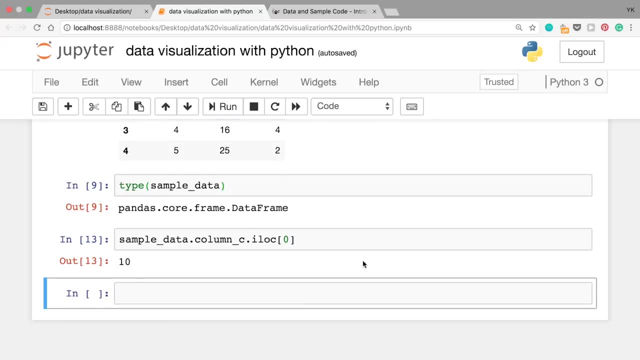 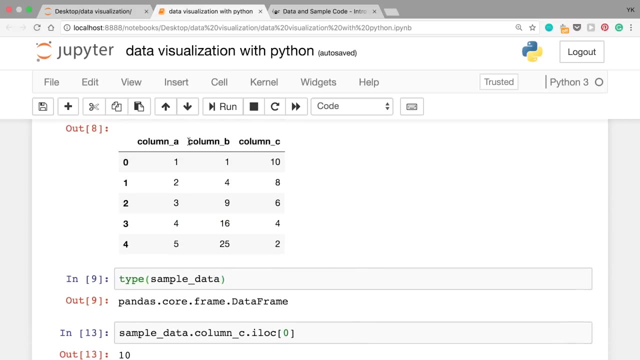 retrieve the first value. you can write iloc 0 and this should give us 10 and it does okay. and using what we've just learned here, we'll be able to plot the data in this data frame. so let's say we want to plot column a on the x-axis and column B on the y-axis. we can do that by: 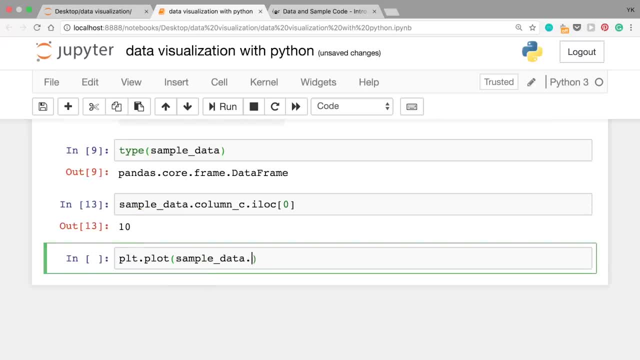 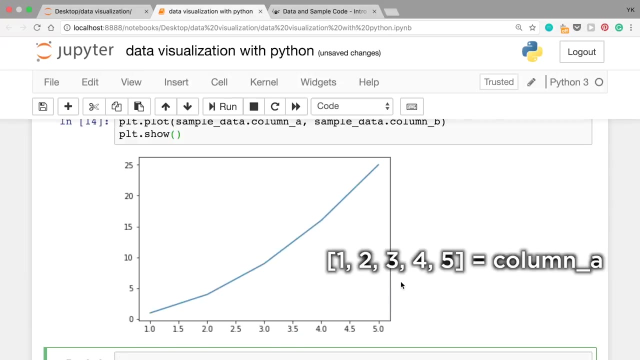 writing PLT that plots sample data dot column a, comma sample data dot column B and we can show it by writing that show. let's see how it looks. we have 1, 2, 3, 4 and 5 on the x-axis and on the y-axis we have 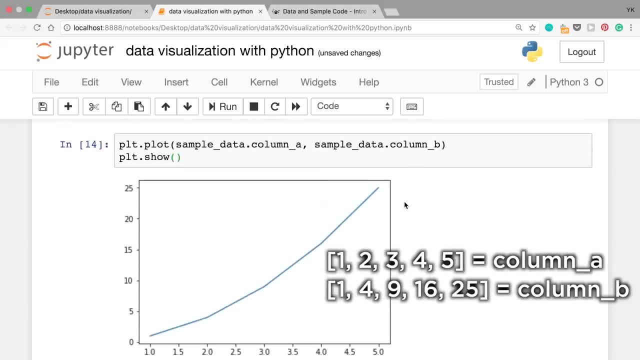 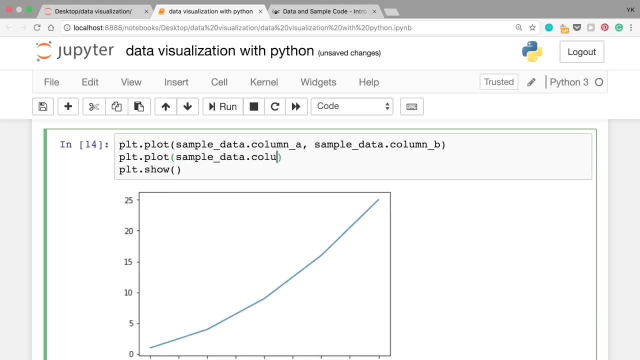 1, 4, 9, 16 and 25, as expected. if you want to add column c to this data, you can write pltplots. sample data dot column a. so let's use column a as the x-axis again and sample data dot column c. 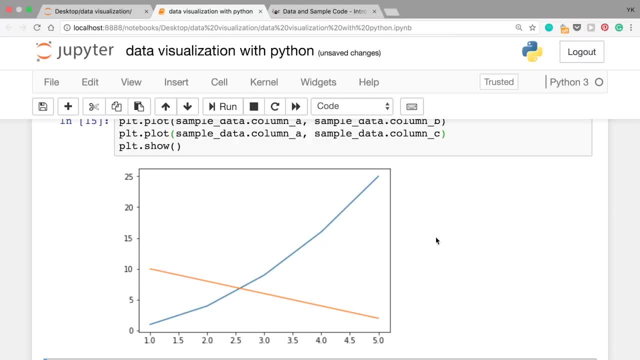 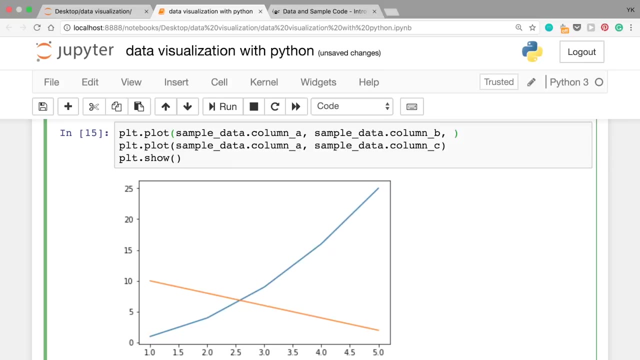 when you run the cell, you see that there are two lines here, just like before. if you want to make this graph a little bit easier to read, you can add the titles and a legend and, by the way, in this plot function you can use the third argument to change how the plot looks. so, for example, if you 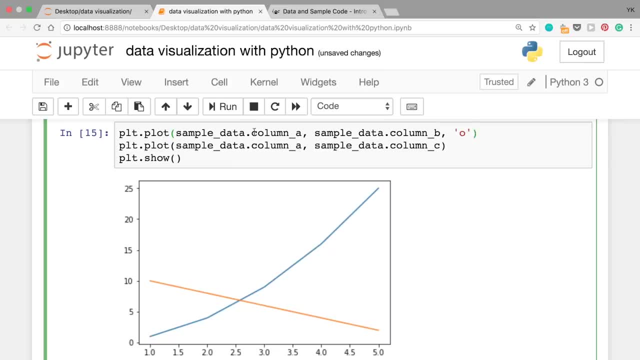 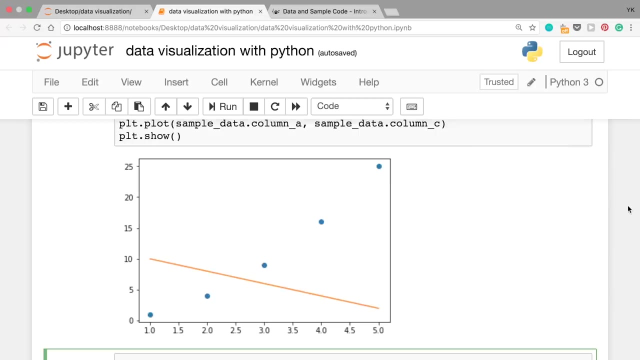 give it o in a string as the argument in the first line for column b, and when you run the cell the plot becomes dots instead of just a line. and there's a lot more you can do if you want to do, and you can find more about it in the official documentation. anyway, let's move on and do, sort of. 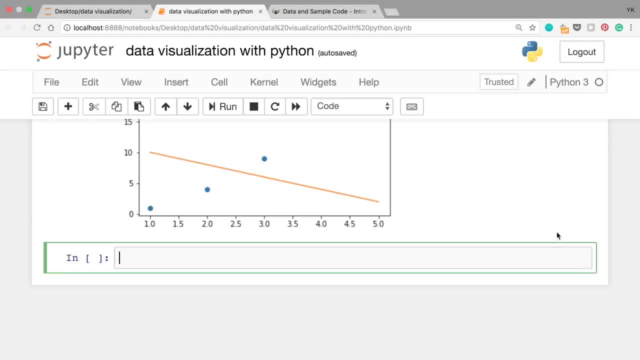 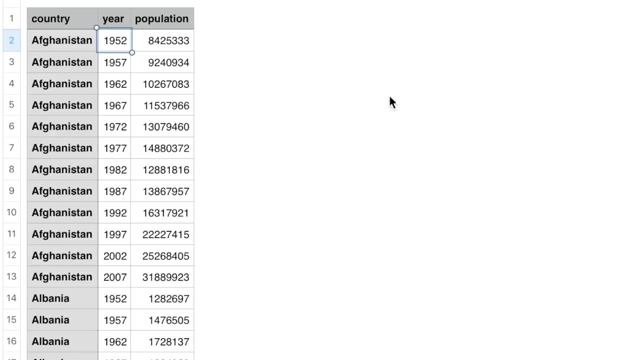 a real analysis with a real data set. now, for this analysis, we're going to use this data: countriescsv. it should be in the same folder as well and when you open it you should see this data. so we have a bunch of countries and a bunch of years, ranging from 1952 to 2007, for every five. 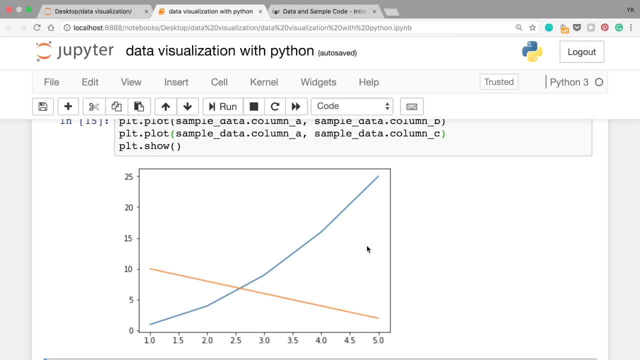 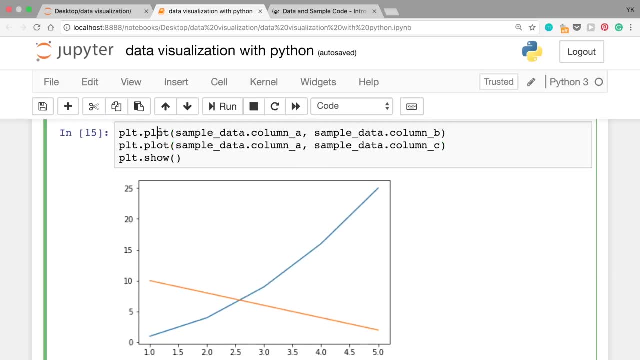 are two lines here, just like before. if you want to make this graph a little bit easier to read, add titles and a legend and, by the way, in this plot function you can use the third argument to change how the plot looks. so, for example, if you give it o in a string as the argument in the first, 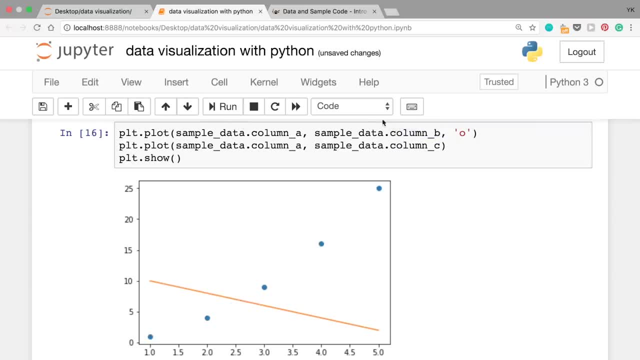 line for column b and when you run the cell the plot becomes dots instead of just a line. and there's a lot more you can do and you can find more about it in the official documentation. anyway, let's move on and do sort of a real analysis with a real dataset. 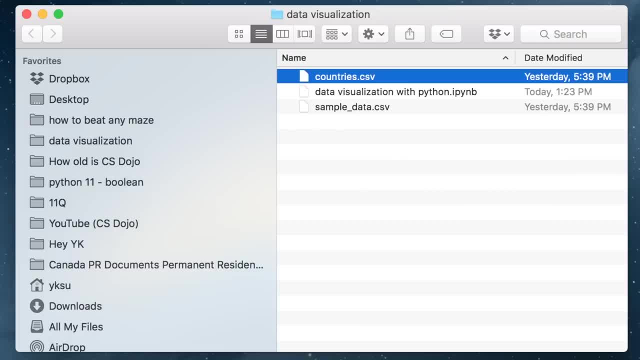 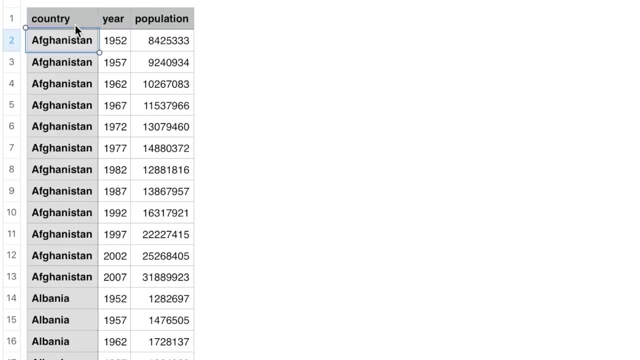 now for this analysis. we're going to use this data, countriescsv. it should be in the same folder as well and when you open it you should see this data. so we have a bunch of countries and a bunch of years, ranging from 1952 to 2007, for every five years, and population for each year for that. 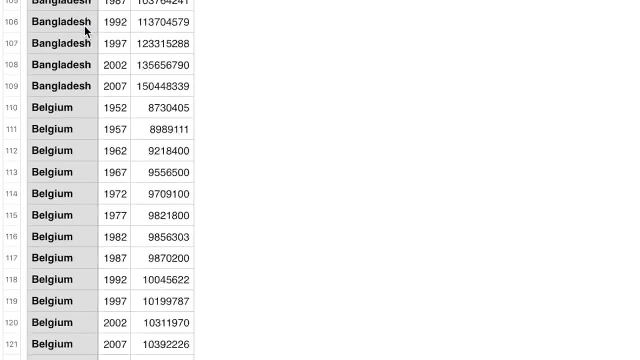 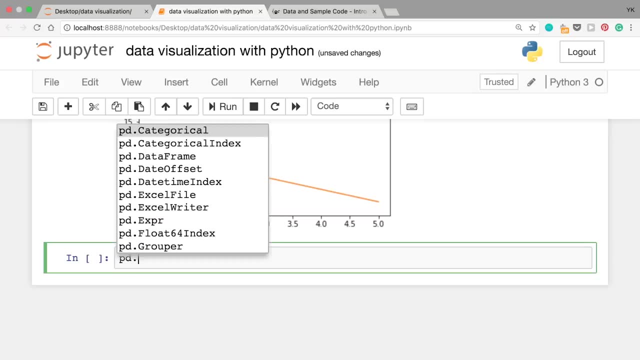 country and you can see that there are a lot of rows in this data. so let's now import that data, just like before by writing pd or panda that read csv, parentheses, single quotes or double quotes, countries that csv. and, by the way, this is a string: single quotes, countriescsv. and in python you can use either double quotes or single quotes. 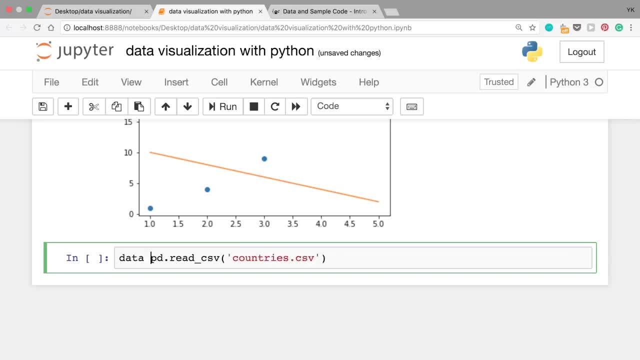 to express a string. let's assign that to a new variable called data. by writing, data equals and when you run this cell, this data is loaded onto data. so once you write data in this new cell and run it, you should be able to see this data cell now in theлушka. perfect and the cooperation between the three cosa windows and same quandato percolator should happen harmoniously. let's say: oh my god, i'll just make sure that the data cells are multiplied monthly. percolator 2. you see that the data system's broken down easily. but let's make it look that way because you can only do these three components. 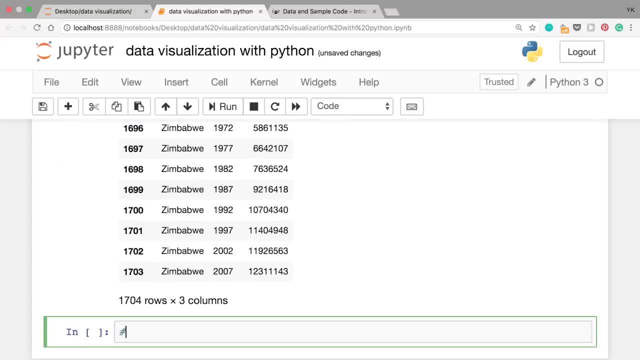 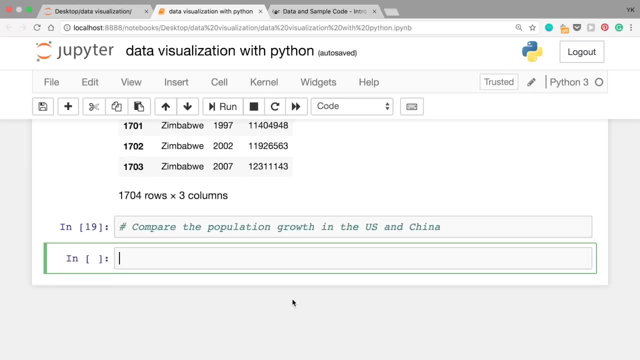 visual porch data essentially of is encountered, and again string and and the loss. what about here, this data in a data frame? now, let's say that the analysis we want to do here is: we want to compare the population growth in the us and china. now to do this analysis, the first thing we want to do 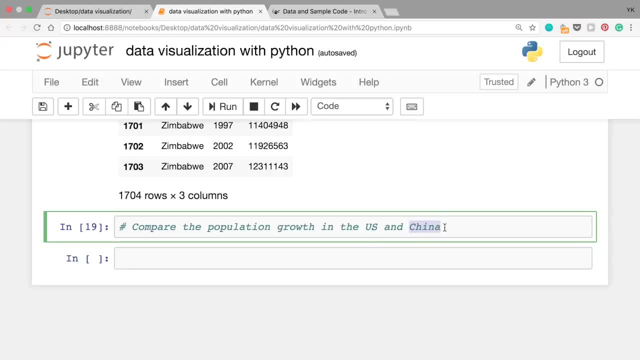 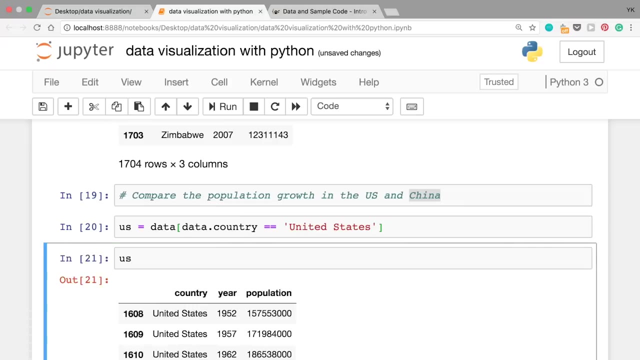 is, we want to isolate the data for the us and china. we can do that for the us by writing: us equals data, square brackets. datacountry equals united states in single quotes, and when you run this cell, us now only contains the data for the united states. so let's break down this statement. 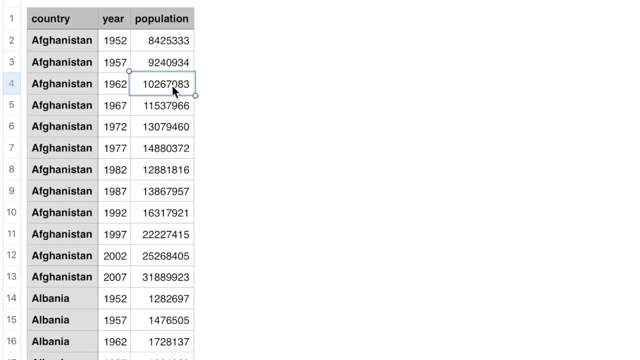 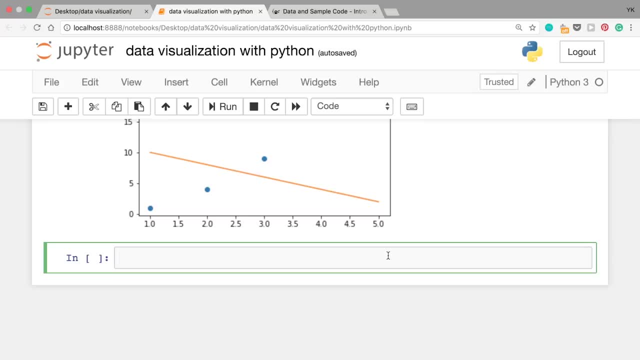 years and population for each year for that country, and you can see that there are a lot of rows in this data. so let's now import that data, just like before, by writing pd or pandas that read csv, parentheses, single quotes or double quotes, countriescsv, and by the 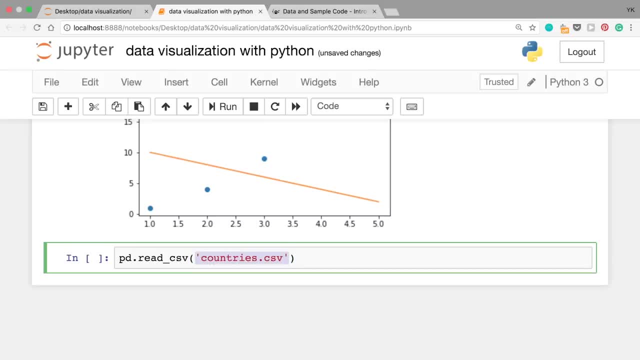 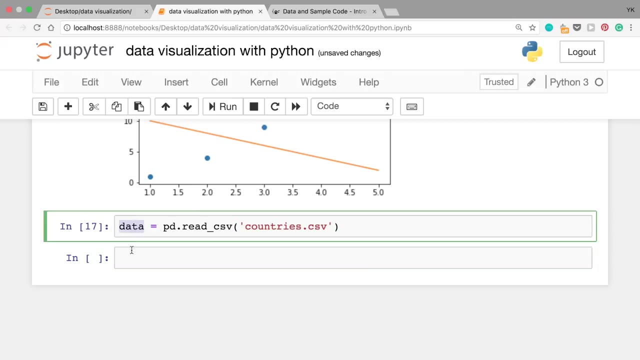 way. this is a string- single quotes- countriescsv- and in python you can use either double quotes or single quotes to express a string. let's assign that to a new variable called data by writing data equals and when you run this so this data is loaded onto data. so once you write data in this new cell and run it, you should be able. 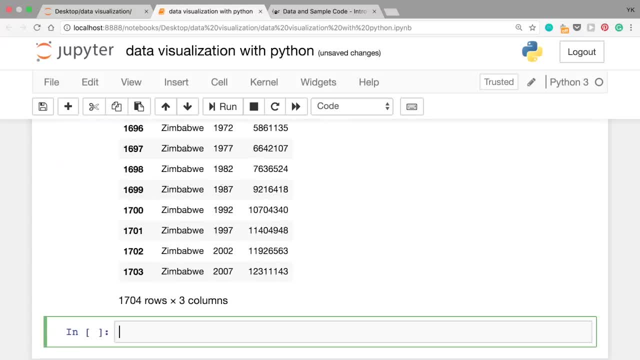 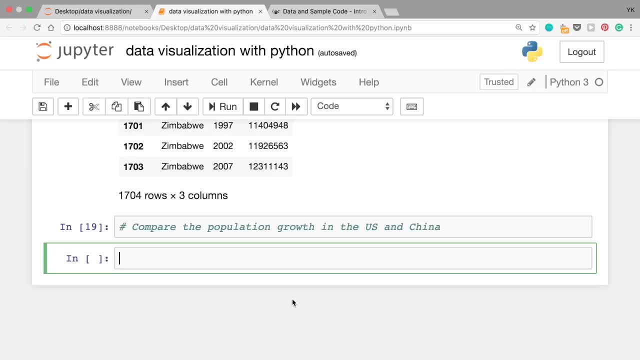 to see this data in a data frame. now, let's say that the analysis we want to do here is we want to compare the population growth in the us and china. now to do this analysis, the first thing we want to do is we want to isolate the data for the us and china. we can do that for the us by writing. 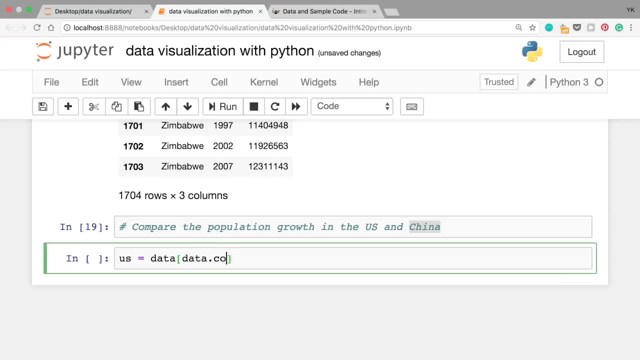 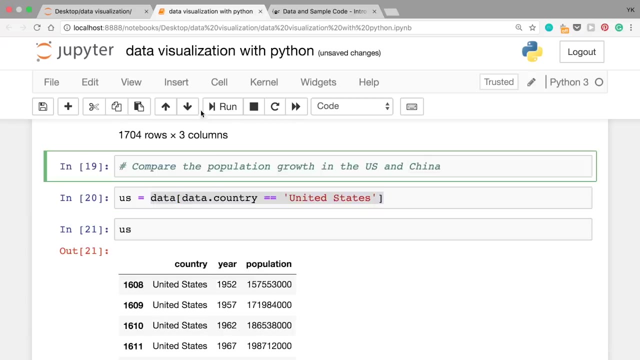 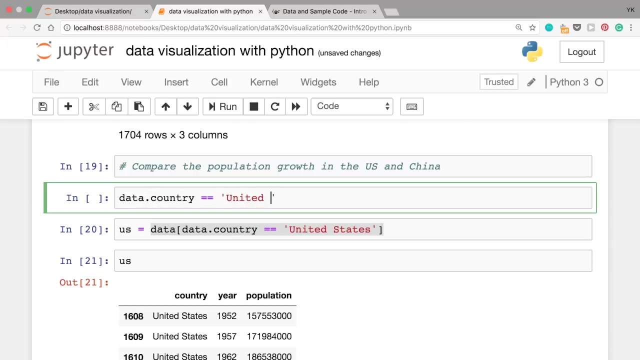 us equals data, square brackets, data that country equals united states in single quotes. and when you run this cell, us now only contains the data for the united states. so let's break down this statement a little bit more. let's click insert here and insert cell below. when you write data that country equals united states, this actually. 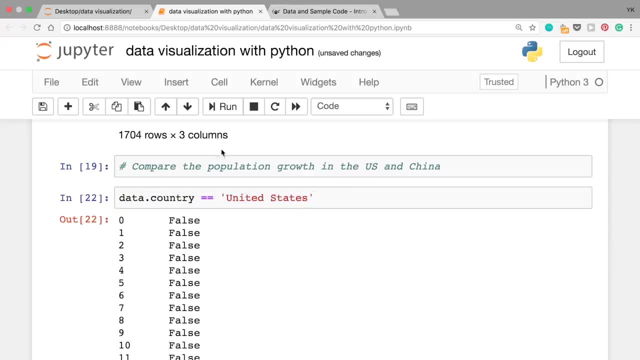 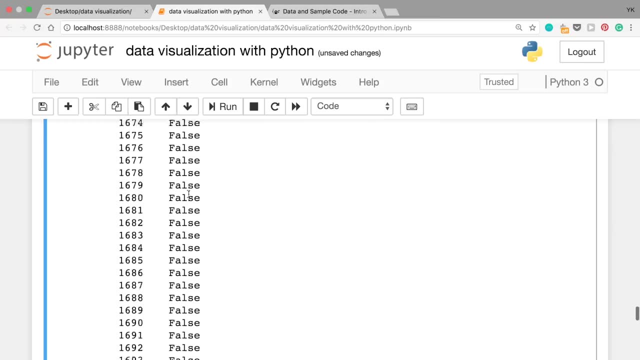 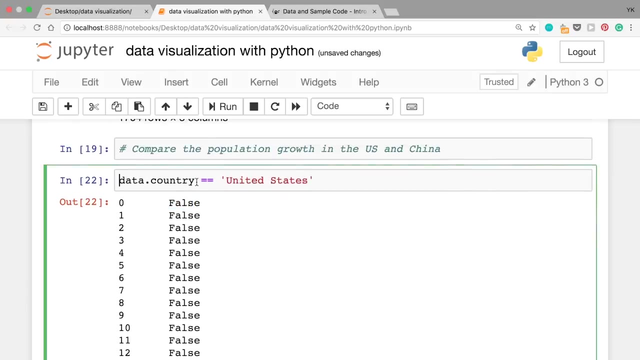 gives a series of a bunch of trues and falses. so when the row is not us, this gives us false, and when it is us, it gives us true. we don't see any trues here, but there are a bunch of trues here where the rows are for the us. and then when you write data square brackets- this a series of bunch. 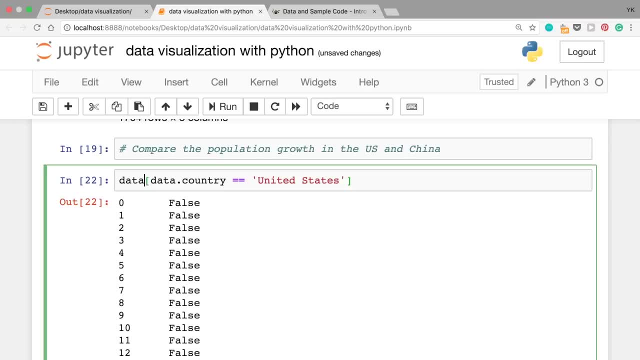 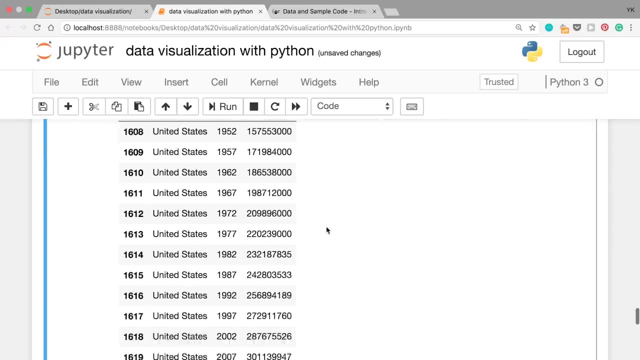 of trues and falses. this gives us a portion of the data where the value of the series is true- and that's the data for the us, as you can see here- and then we just assign it to this variable called us. okay, let's now do the same thing for the second data. 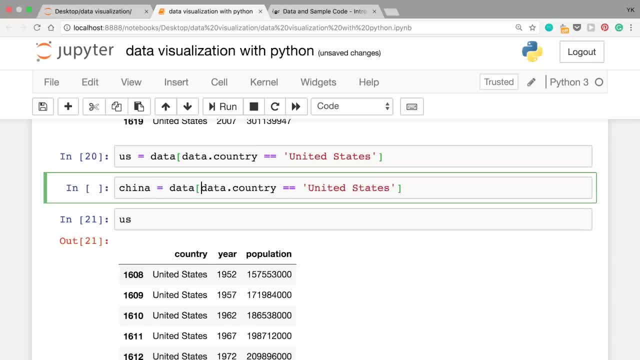 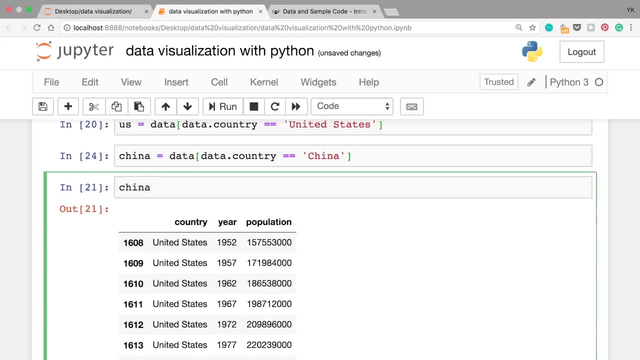 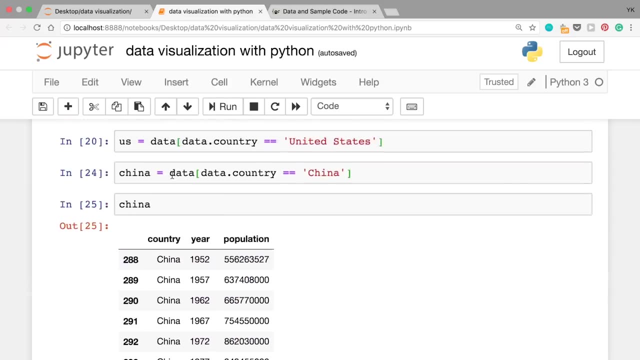 for China by writing: China equals data, square brackets- datacountry equals China, and when you run this cell and when you write China here and run this cell, you should only see the data for China and using these two variables, US and China will be able to compare their. 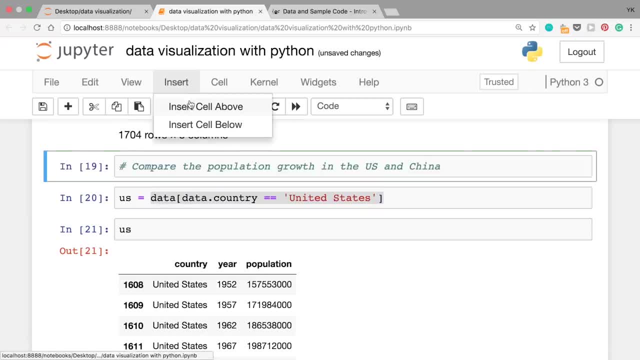 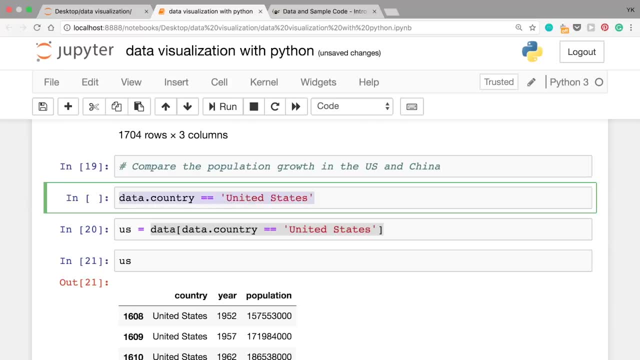 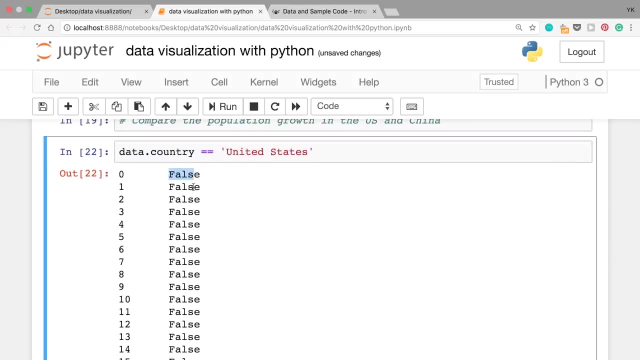 a little bit more. let's click insert here and insert cell below. when you write, datacountry equals united states, this actually gives a series of a bunch of trues and falses. so when the row is not us, this gives us false, and when it is us, it gives us true. we don't see any trues here. 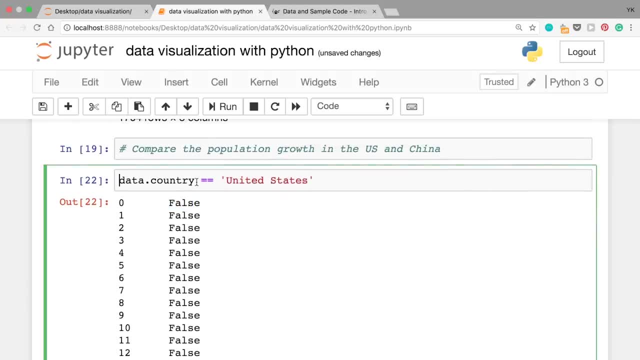 but there are a bunch of trues here where the rows are for the us, and then when you write data, square brackets, this a series of bunch of trues and falses. this gives us a portion of the data where the value of the series is true and that's the data for the us, as you can see here. and then 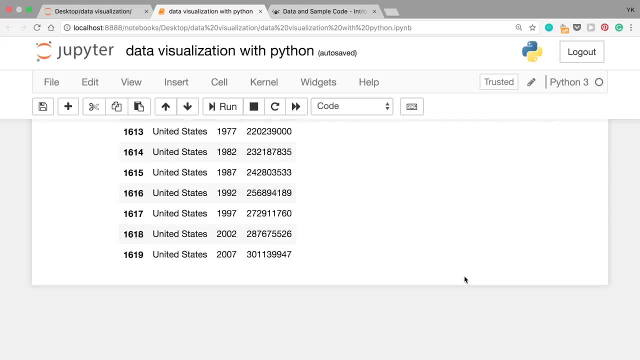 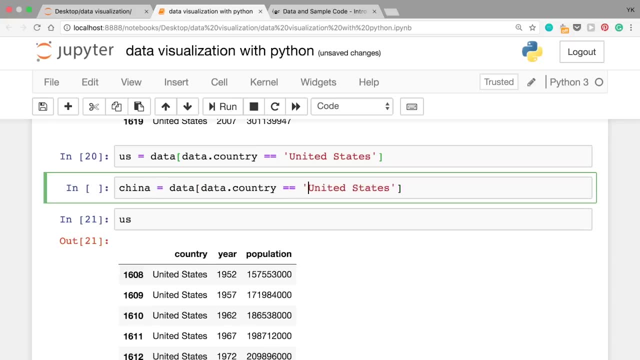 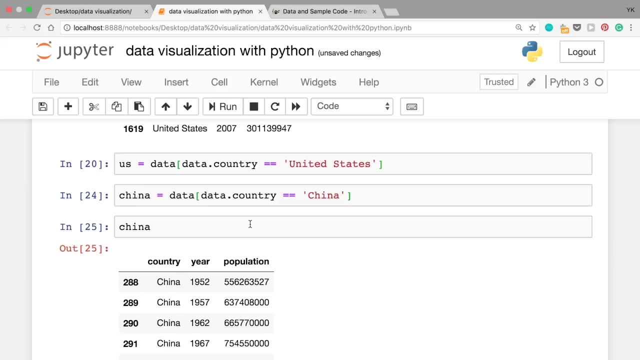 we just assign it to this variable called us. okay, let's now do the same thing for china. by writing china equals data, square brackets, data country equals china, and when you run this cell. and when you write china here and run this cell, you should only see the data for china. and using these two variables, us and china will be able to. 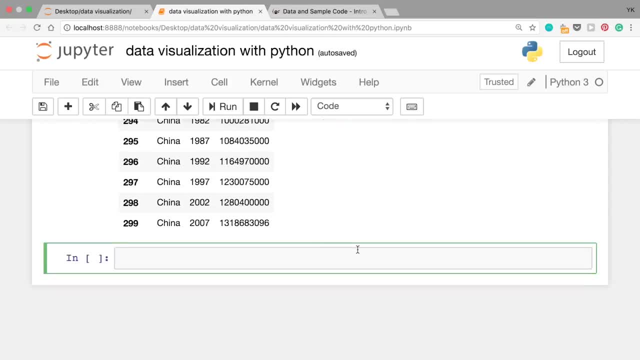 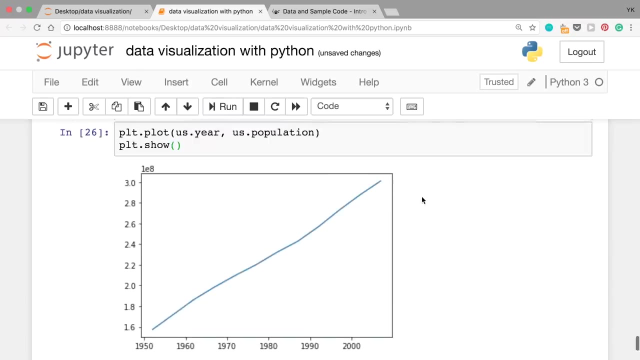 compare their population growth. so let's first plot us's population here by writing pltplot- usyear comma- uspopulation. you can show this plot with pltshow and when you run this cell you should see this graph. you see that usyear is plotted on the x-axis and uspopulation is plotted on the y-axis. 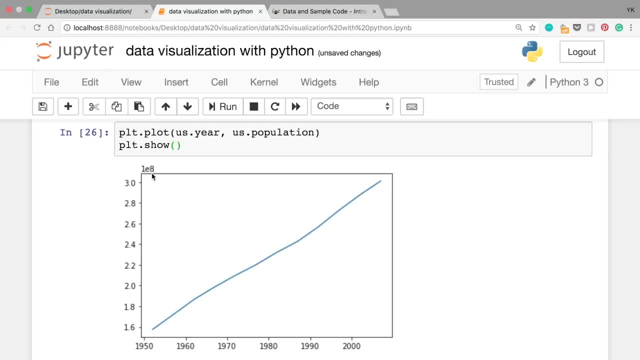 but you see this scientific notation thing, 1e8, because the numbers are so big. so let's divide the whole population, each number in the series, with 1 million, or 10 to the power of 6, that's 10 star star 6 in python. and when you run this cell again you now see the population in millions. 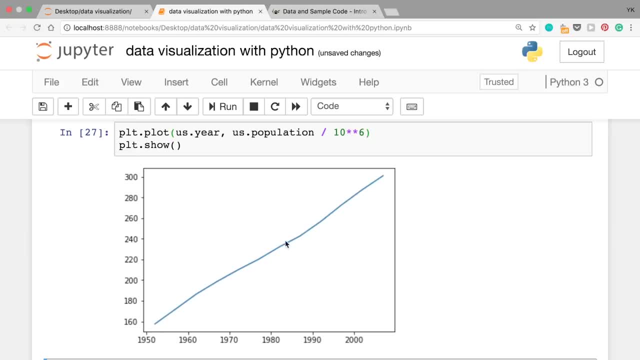 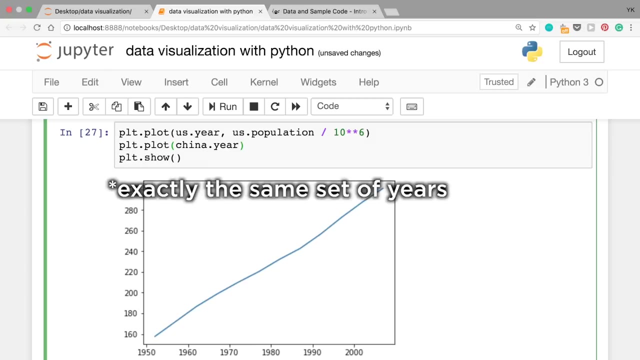 so this is 160 million and it goes up to, i think, more than 300 million in 2007.. and let's plot china's data on top of this plot by writing pltplot: chinayear. actually, you could use usyear or chinayear, because we have exactly the set of years, but for now let's just use chinayear for the x-axis and 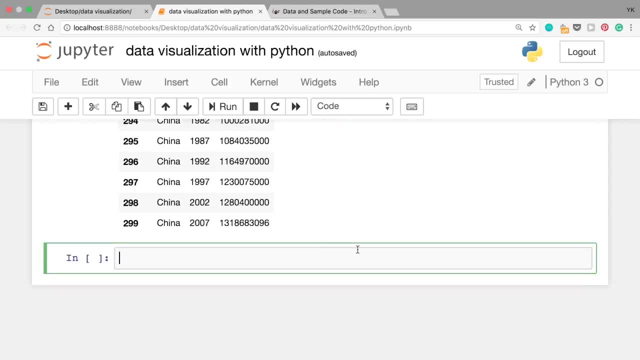 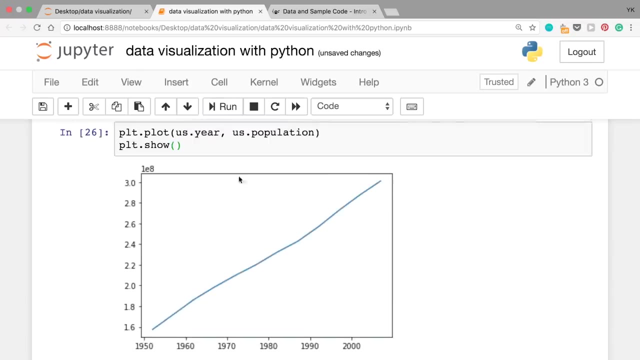 population growth. so let's first plot US's population here by writing pltplot- usyear comma- uspopulation. you can show this plot with pltshow and when you run this cell you should see this graph. you see that usyear is plotted on the x-axis and uspopulation. 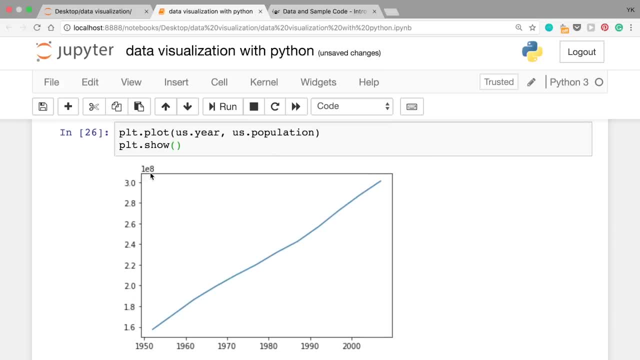 is plotted on the y-axis. but you see this scientific notation thing, 1e8, because the numbers are so big. so let's divide the whole population, each number in the series, with 1 million, or 10 to the power of 6, that's 10 star star. 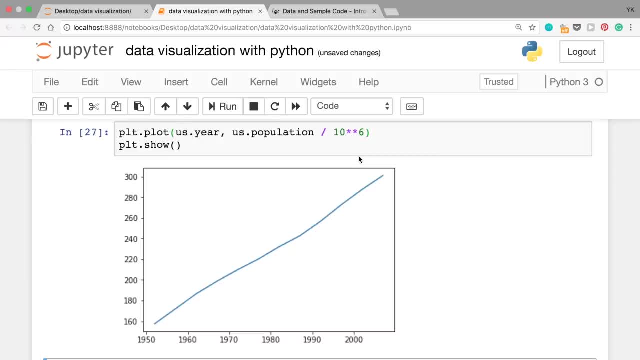 6 in Python, and when you run this cell again, you now see the population in millions. so this is 160 million and it goes up to, I think, more than 300 million in 2007. and let's plot China's data on top of this plot by writing pltplot- Chinayear. actually you could use 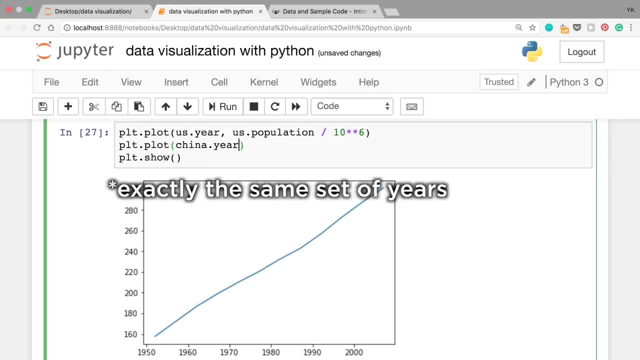 usyear or Chinayear, because we have exactly the same of years, but for now let's just use Chinayear for the x-axis and usyear for the y-axis, and we're going to divide this by 1 million as well to make the population show in millions, and when you run the cell you should see these two lines. let's. 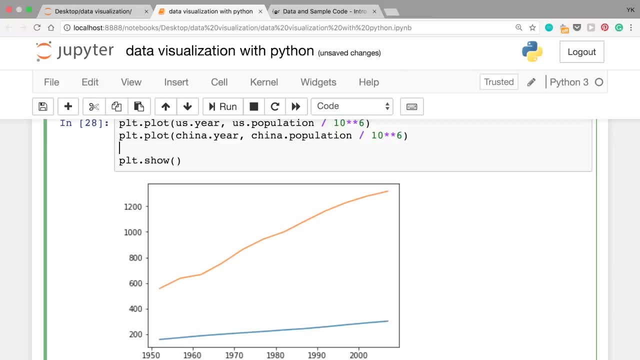 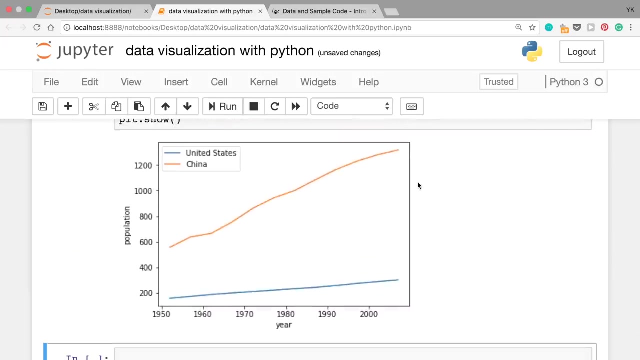 add a legend and titles here to make this graph easier to read. so pltlegend parentheses, square brackets, United States and China, and the x label- pltxlabel- should be just year and the y label should be population. run this cell again and this graph is much easier to. 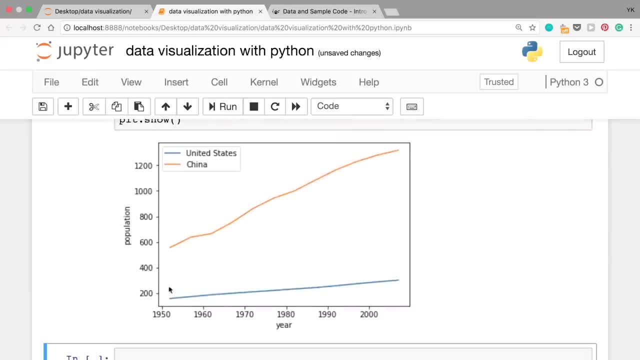 read, so you can see that China's population started out much larger than the US in 1952, and it seems like it's going faster as well now. what if you wanted to compare, instead of the absolute amount that you see here, the percentage growth from the first year that? 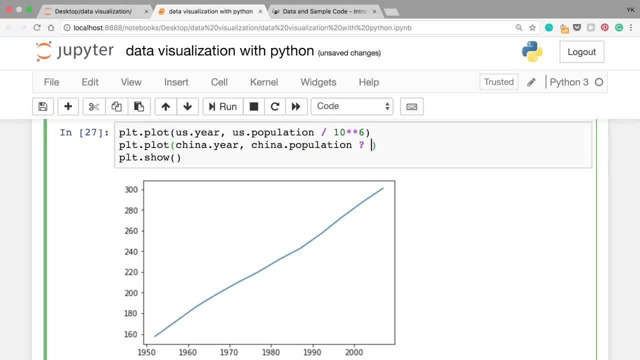 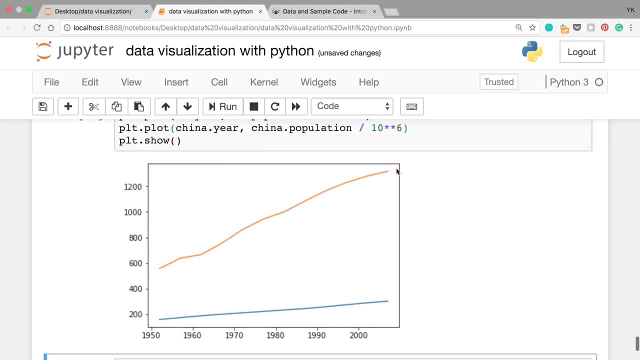 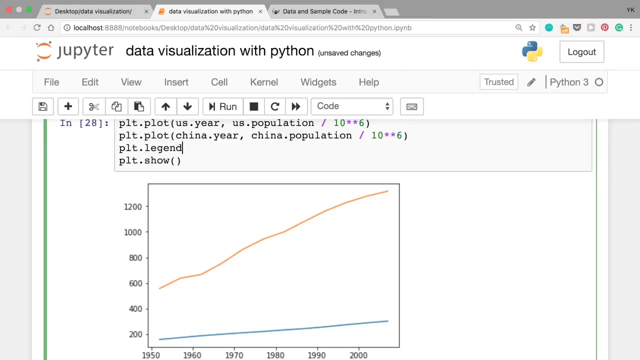 china dot population for the y-axis and we're going to divide this by 1 million as well to make the population show in millions, and when you run the cell you should see these two lines. let's add a legend and titles here to make this graph easier to read. so pltlegend parentheses, square brackets. 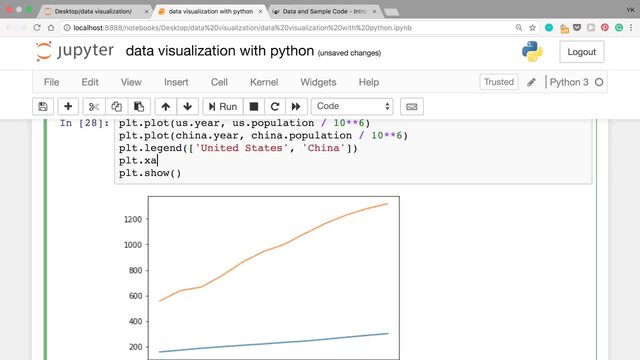 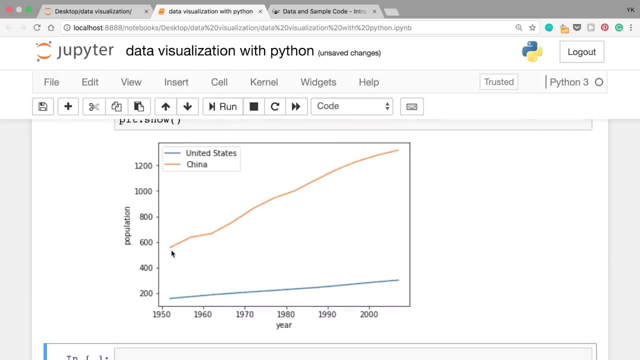 united states and china and the x label, pltx label should be just here and plty label should be population. run this cell again and this graph is much easier to read so you can see that china's population started out much larger than the us in 1952 and it seems like. 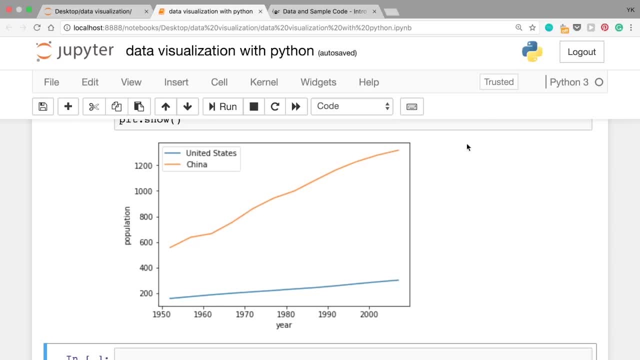 it's going faster as well. now, what if you wanted to compare, instead of the absolute amount that you see here, the percentage growth from the first year that we have in our data, 1952? well, there are several different ways of doing this, but i'm going to show you just one way so to do that. 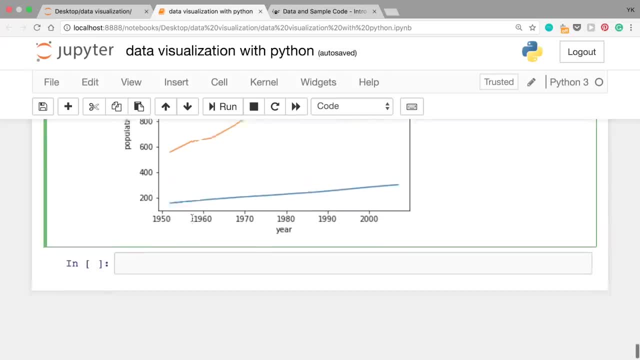 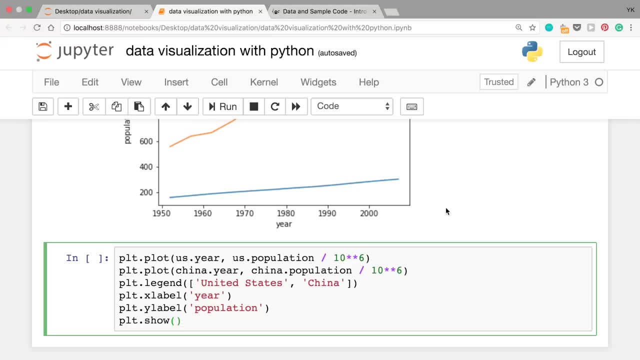 let's first copy this whole block of code over here and let's say that for each country we want to find the percentage growth from the first year. so we want to set the first year's amount to 100 as in 100 and show the rest of the data in percentage relative to the first year and 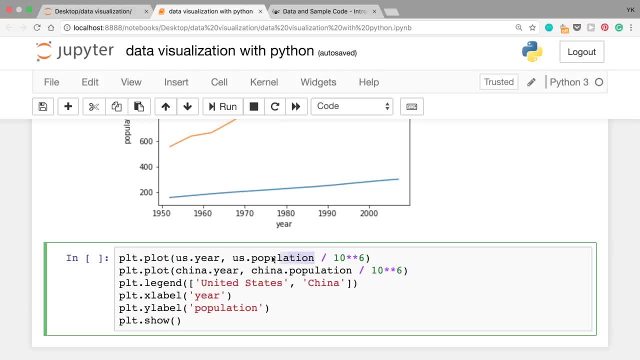 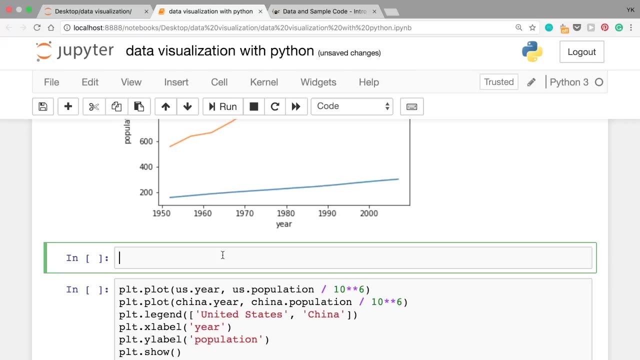 we can do that by dividing this whole series, for example usd population, with the first year's population and then multiplying everything by 100.. so to show you how to do that, you need to create a new cell here above by clicking insert cell above, here and here first i'm going to write. 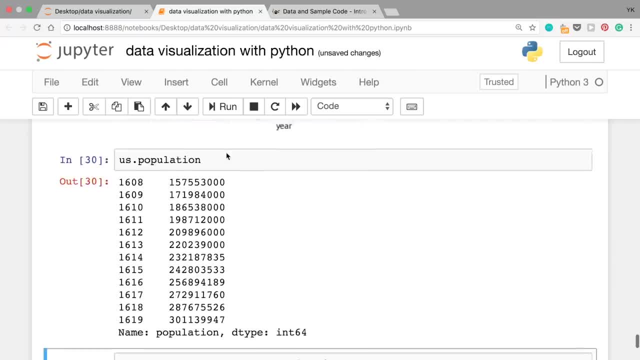 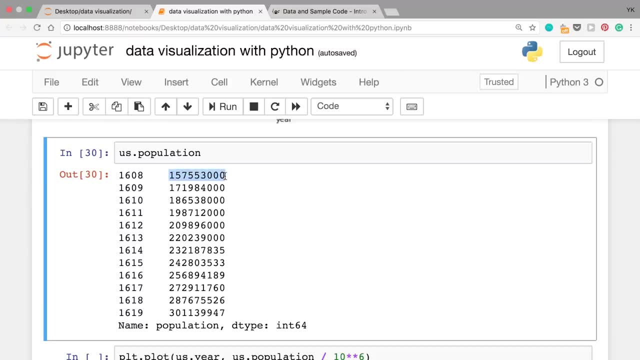 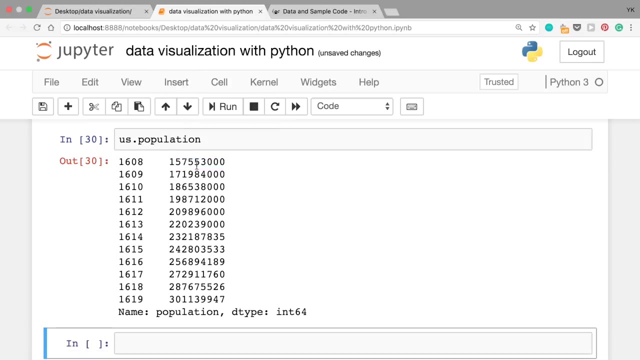 us dot population and you see a series of population here for each year and the first row you see here is the first year's population, or the population in 1952, i think, and let's insert a new cell below here now to retrieve the first year's population you can just write uspopulation. 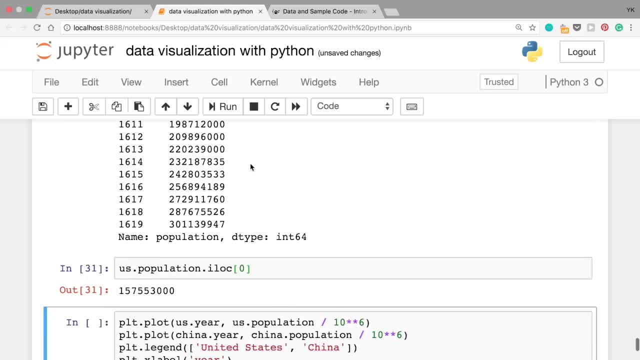 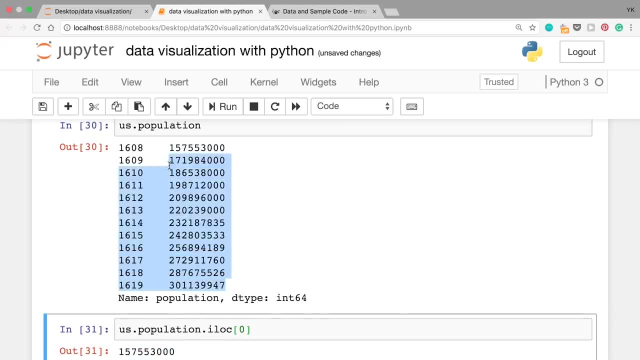 dot iloc, square brackets zero, and this gives us the first year's population, which is this amount. then we can divide the whole population, this whole series, by the first year's population, just by writing: uspopulation divided by uspopulation: dot iloc, square, brackets, zero, and this gives us: 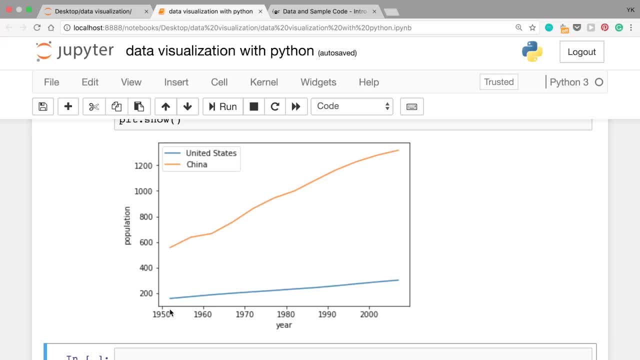 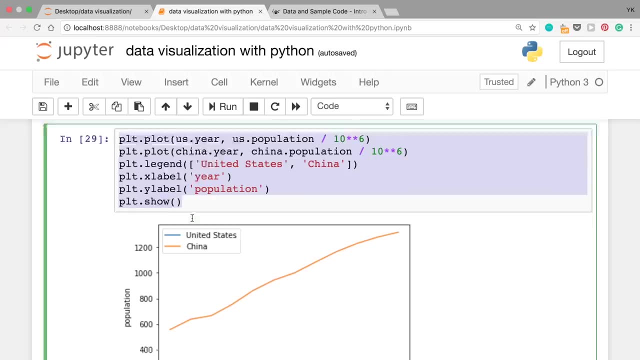 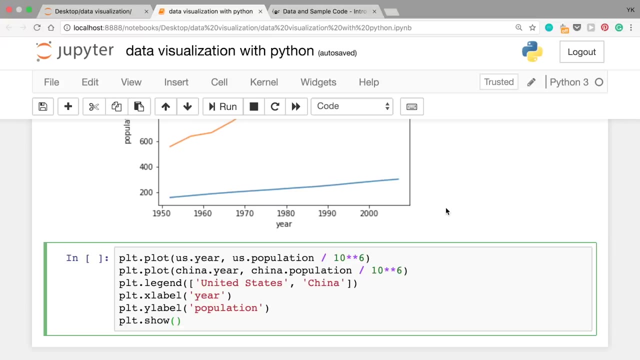 we have in our data 1952. well, there are several different ways of doing this, but I'm going to show you just one way. so to do that, let's first copy this whole block of code over here and let's say that for each country, we want to find the percentage growth from the first year. so we want to set 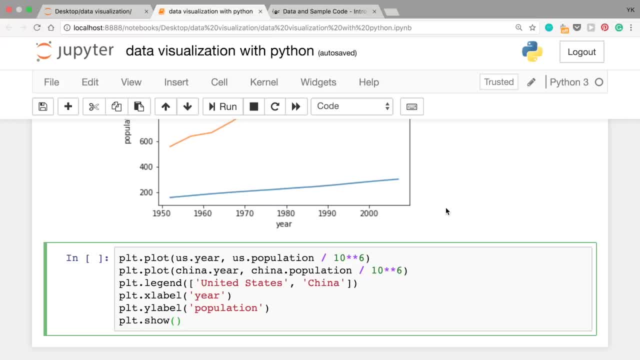 the first year's amount to 100, as in 100 percent, and show the rest of the data in percentage relative to the first year. and we can do that by dividing this whole series, for example uspopulation, with the first year's population and then multiplying everything by 100. so 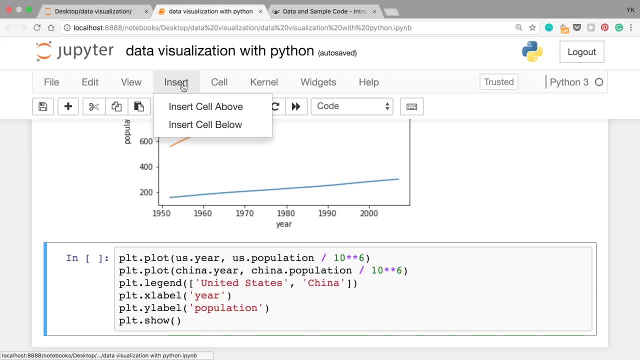 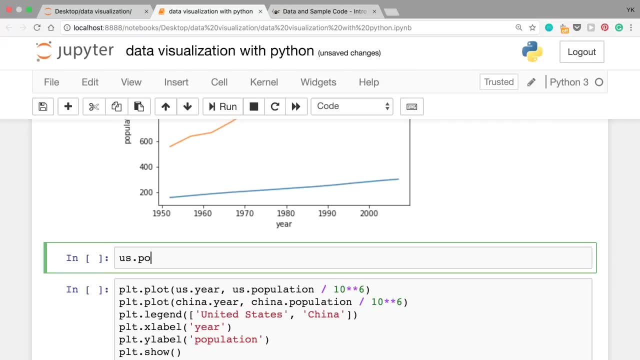 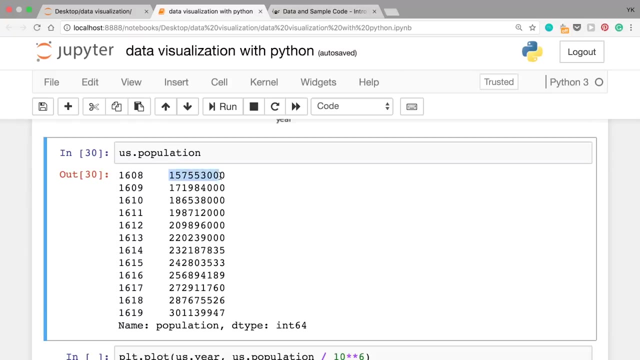 to show you what I mean, let's just create a new cell here above by clicking insert cell above. here and here first I'm going to write uspopulation and you see a series of population here for each year and the first row you see here is the first year's population or the 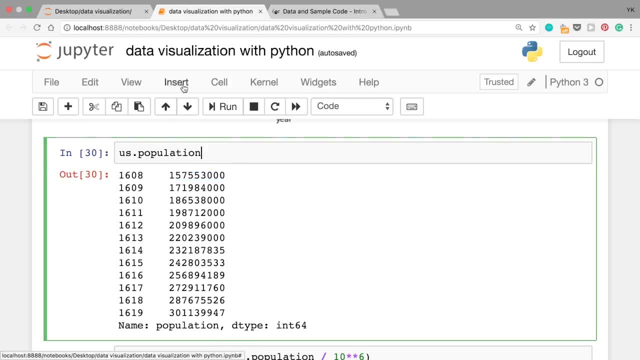 population in 1952, I think, and let's insert a new cell below here now to retrieve the first year's population. you can just write uspopulation. so in fact I'm going to create a new cell here and let's see the results here. so the first year's population for the 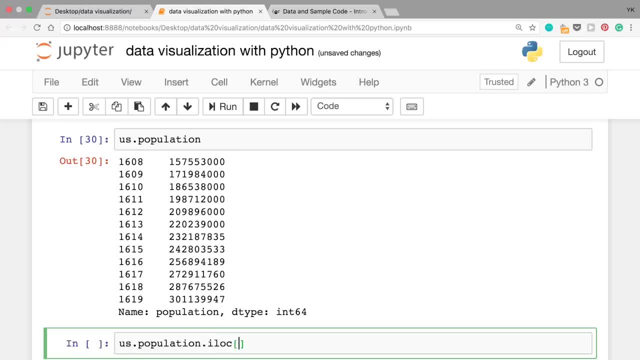 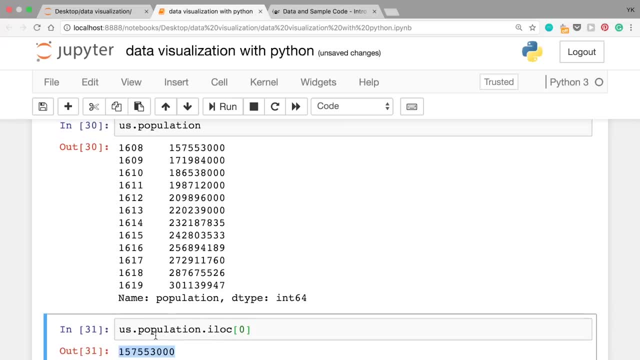 first year's population is 100 and it's actually less than the previous year's population. so population dot, iloc, square brackets, zero, and this gives us the first year's population, which is this amount. then we can divide the whole population, this whole series, by the first year's population. 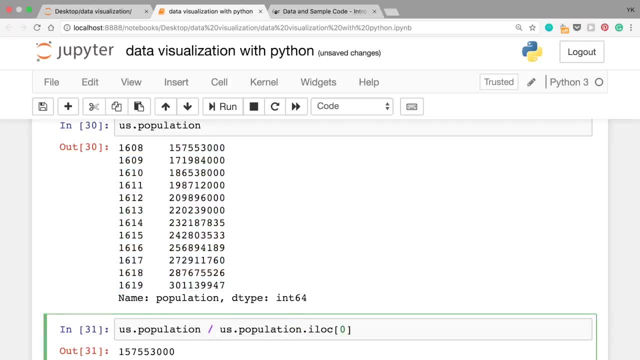 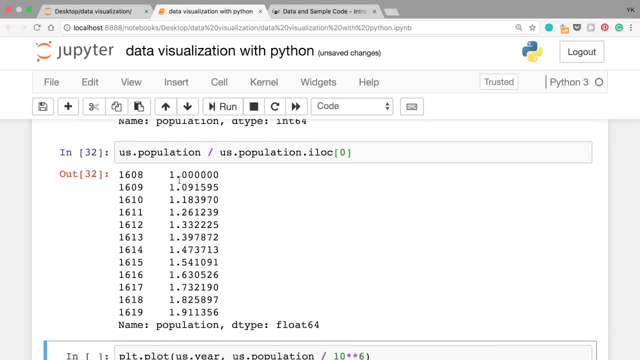 just by writing us dot population divided by us dot population dot iloc square brackets zero, and this gives us this series. so, as you can see, the first year is set to one and the rest of the years are shown in relative amounts. and if you multiply everything by 100, just by writing star. 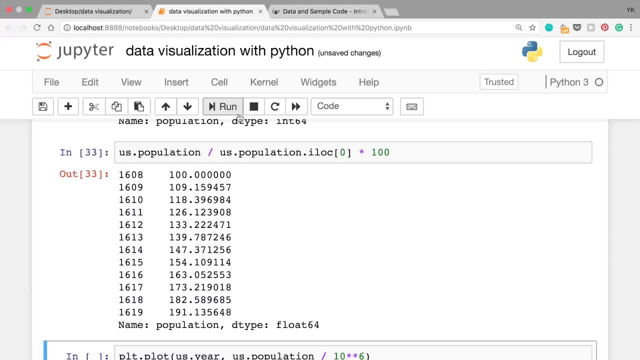 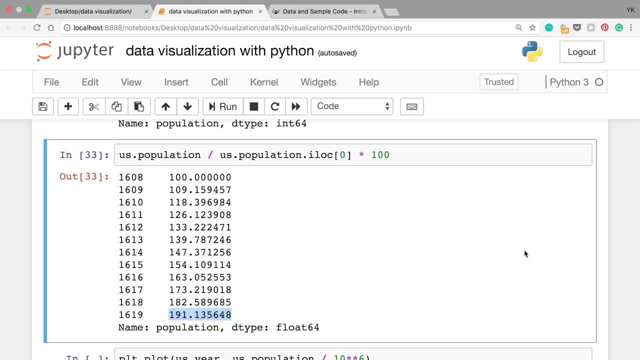 100. here you'll be able to show everything in percentage amounts, so you can see that the first year is shown as 100 and from 1952 to 2007, which is the last year we have, the population grew by 90. now, like i said earlier, this is not the only method to show the relative growth in population. 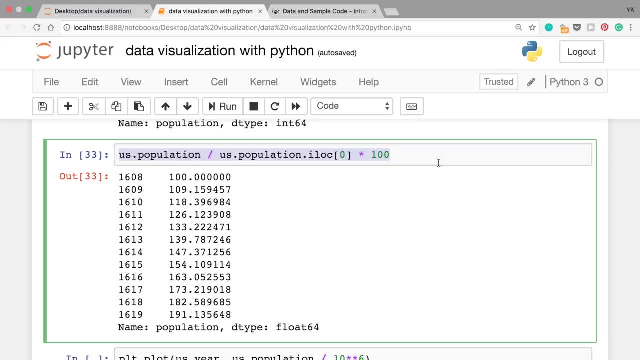 but i chose this method here because it's pretty simple and it's not the only method to show the relative growth in population. but i chose this method here because it's pretty simple and it's not the only method to show the relative growth in population, but i chose this method here because it's pretty simple to implement. 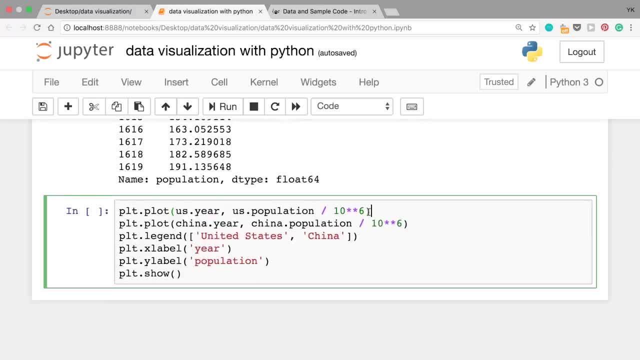 anyway, let's copy this whole thing and paste it over here to replace the y-axis, and let's do the same thing for china as well. so copy the whole thing for china here and then replace us with china. once you do that, let's change the population in y-label to population. 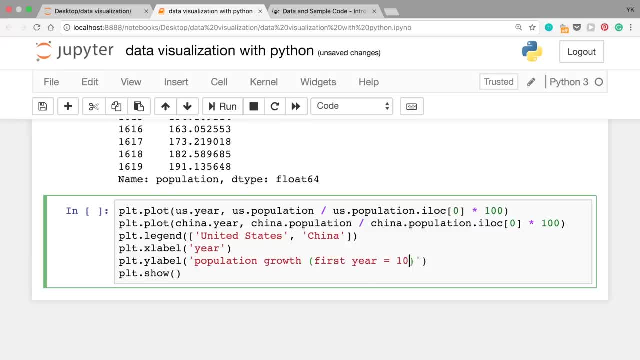 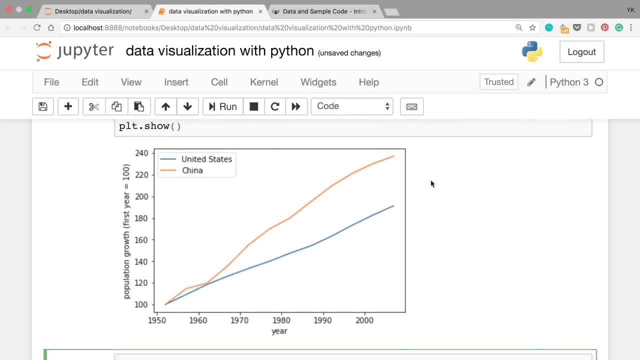 growth- and let's just write first year equals 100, just for clarity here. and when you run this cell, you should see this graph. you should see this graph so you can see that, even in percentage amount, china's population grew much faster than that of united states. the us population grew by 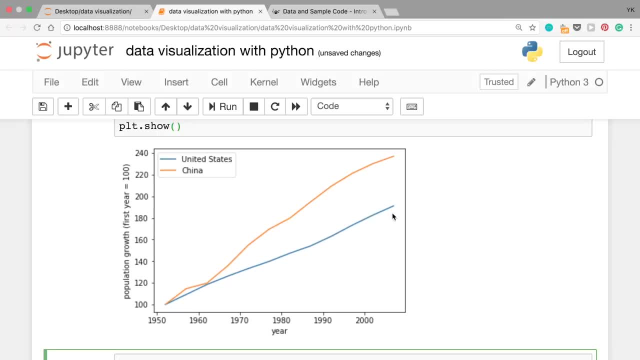 90 from 1952 to 2007.. but during the same time, china's population grew by more than 120 percent. okay, this was a pretty simple example and it actually came from my course called introduction to data visualization. if you like this video, i'd actually highly recommend it. it's a course with more. 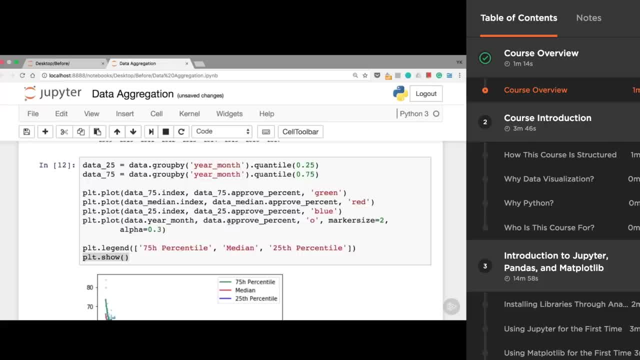 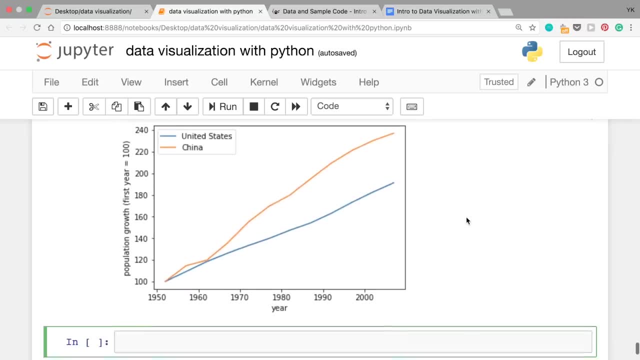 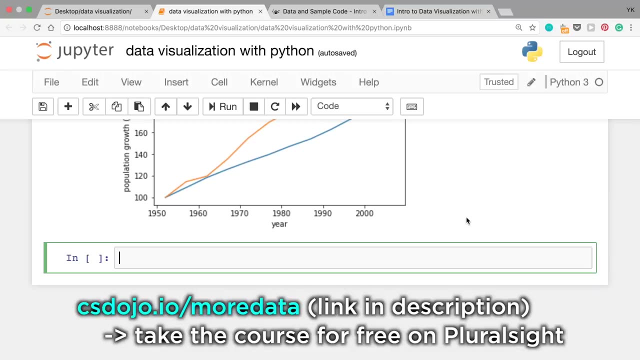 more videos just like this one, and I cover more realistic and complex examples and more different types of data visualization techniques, not just line charts. So if you want to check out the course, you can just go to csdojoio slash more data. You can actually take this course for free by signing. 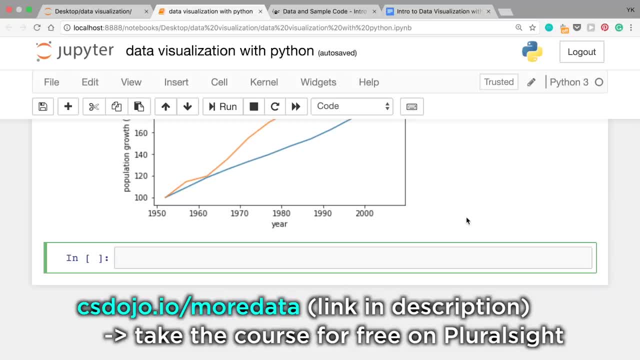 up to Pluralsight's 10-day free trial. That's the site the course is hosted on. Anyway, as always, thanks for watching this video and I'll see you in the next one. 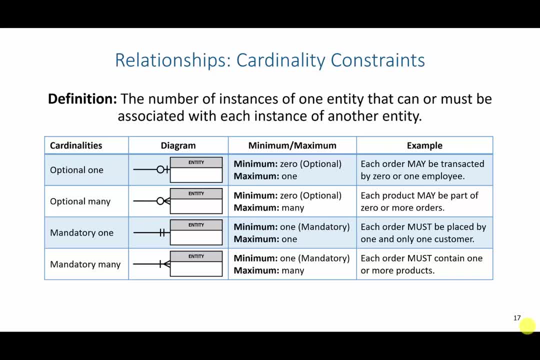 In this video we're going to continue with relationships, specifically looking at cardinality constraints. So cardinality constraints are the number of instances that one entity can or must be associated with each instance of another entity. So take, for example, if I had a entity. 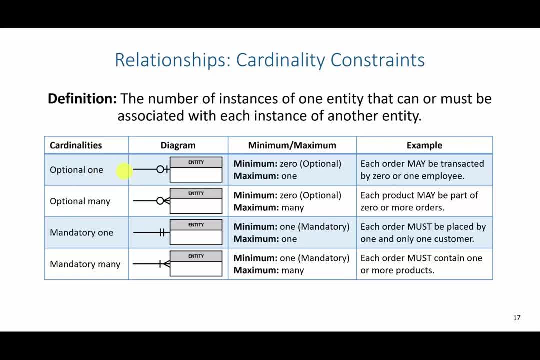 here on the left, with an optional one: cardinality. each instance in that entity would be associated with zero or one instance of this entity. So optional is represented using an O and this line represents one. So in this case our minimum is going to be zero and our maximum is going to.